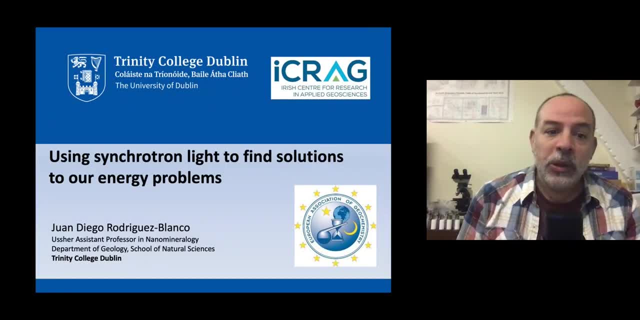 Hello and welcome to this talk about synchrotron radiation and how this radiation can be very useful to find solutions to our energy problems. My name is Juan Diego Rodríguez Blanco and I am a lecturer in nanometeorology at Trinity College study. 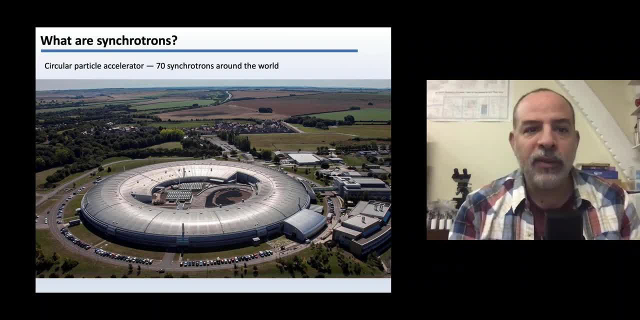 So I'd like to start this talk by giving you some background information about synchrotrons, in case you have never been to one of these facilities. So these are circular particle accelerators and they are very complex facilities. They are very useful because they can produce very intense X-rays and, as you can imagine, 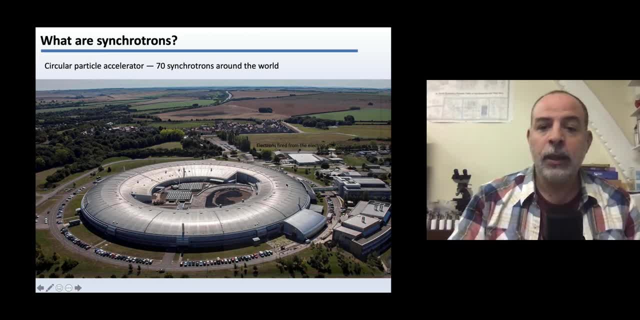 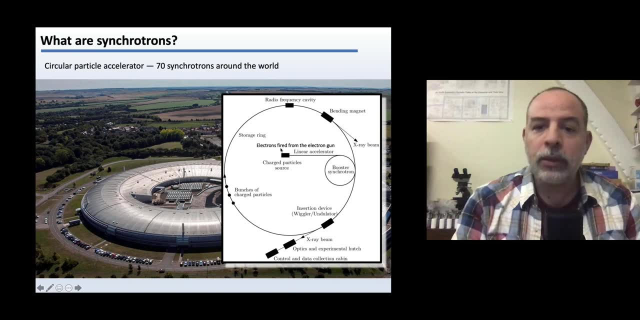 they are so complex that there are less than 100 in our planet. The way they work is by firing electrons from an electron gun here, and they are moving through a linear accelerator, then injected into a booster synchrotron, and here they. 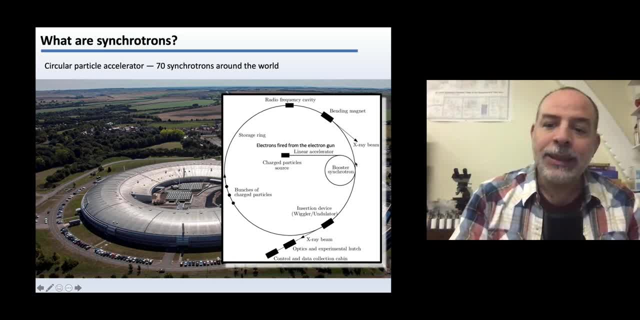 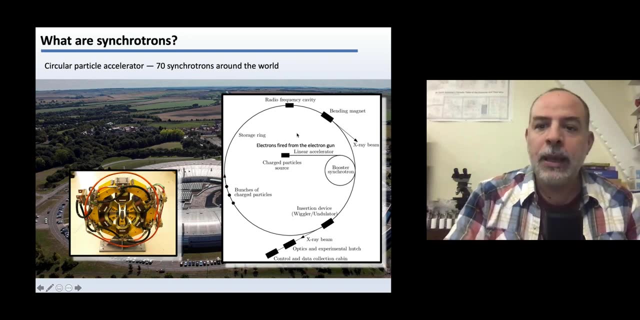 increase their energy And once they have the desired energy, they are injected into the system, Into this bigger ring named the storage ring. Here they move in a circular pathway and this is being done by using bending magnets like these sextuple magnets here. 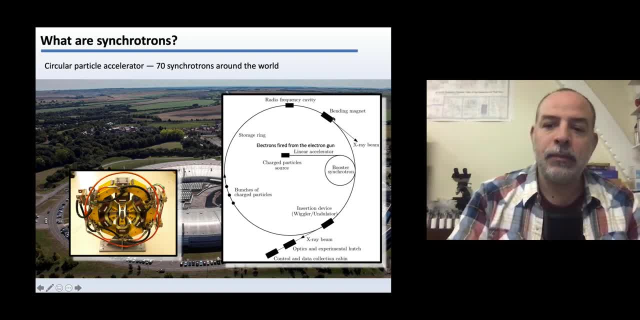 And when they are moving, when the electrons are moving in these circular trajectories, they emit X-rays. These are the X-rays that we use to carry out our experiments. Of course, synchrotrons can produce radiation in our wavelength, So they can produce radiation in our wavelength. 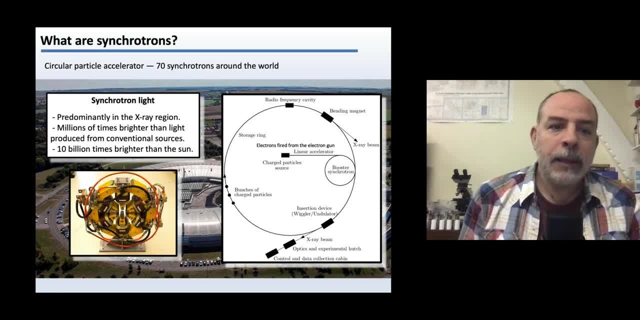 For example, in the ultraviolet or infrared. But most of the research is being done in the X-ray region because this is very useful to understand the nature of matter. These X-rays are brighter than any conventional source, for example, much brighter than the. 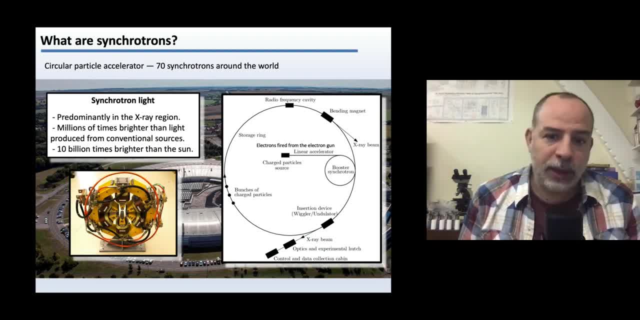 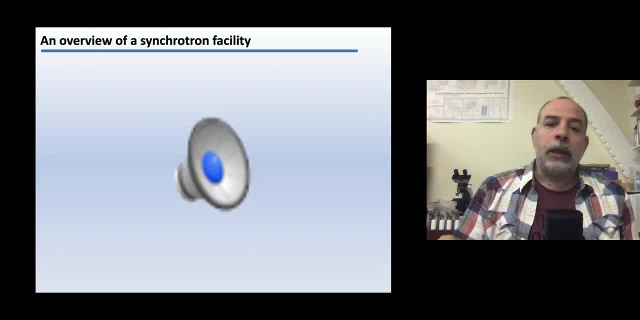 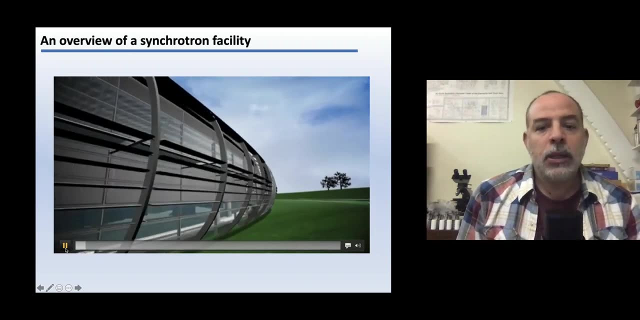 typical single crystal or powder X-ray diffraction systems and also billions of times brighter than the sun. All right, I'm going to show you here A diagram, an animation showing you how a synchrotron works. So this represents a diamond light source which is in the UK, in Oxfordshire. and what 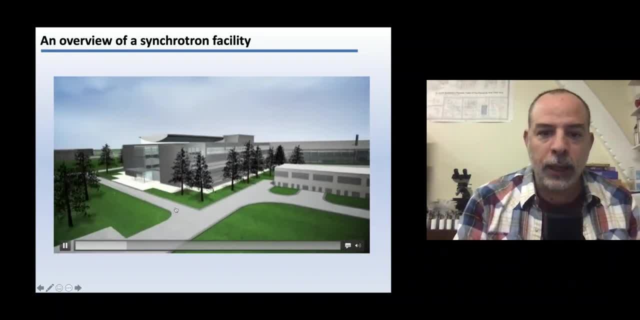 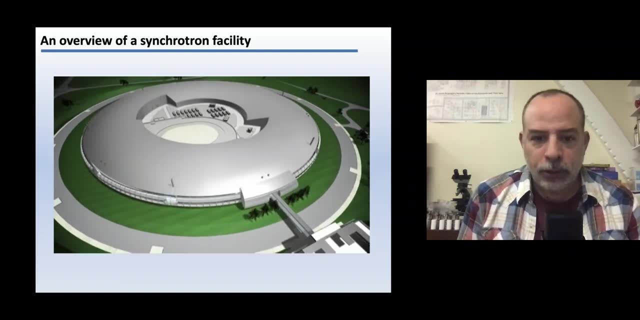 you can see. first, this is a building where the control room is located Here. this is where all the facility is controlled by engineers, and what happens inside the synchrotron is something that you are going to see now and you will see here the gun. 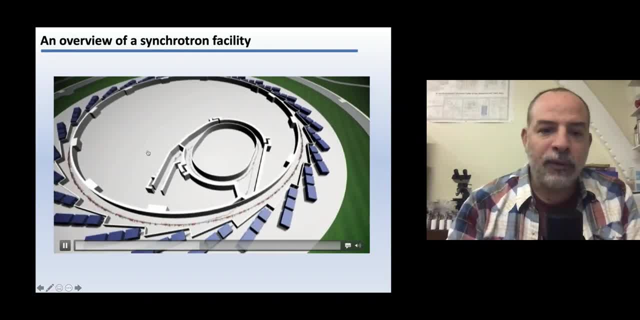 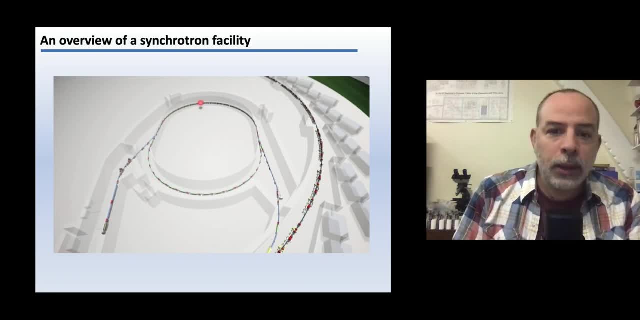 producing electrons And how these electrons act And how these electrons act. So these electrons are fired into this booster ring first, OK, And when the electrons are fired and they are injected into the booster ring, they are accelerated, they reach the desired energy, and after that they are injected into the 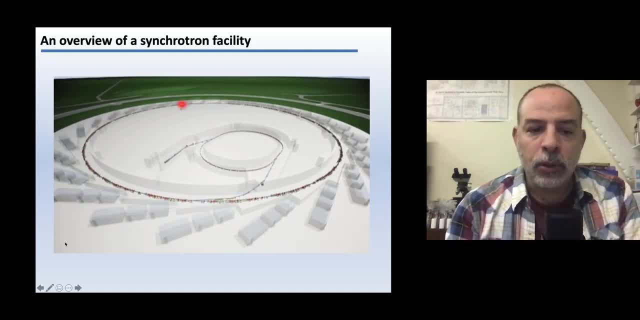 bigger storage ring, And here this is where they produce X-rays. So I'm going to stop the animation, just to tell you a couple of things more. OK, Along all this ring you have different stations to work. They are named beam lines. 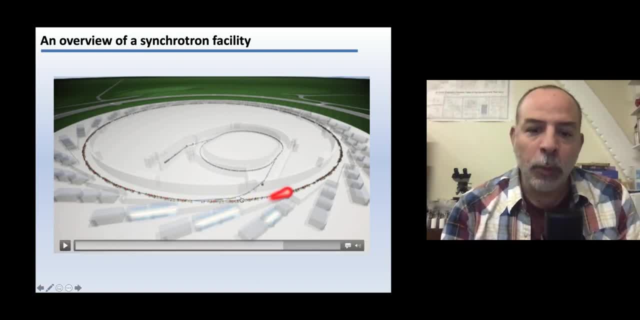 And each beam line is made of three components. First one is an optic hatch. this is where the X-rays are focused. Second one is an experimental laboratory. this is where you carry out your experiments. And the third one is a control cabin. 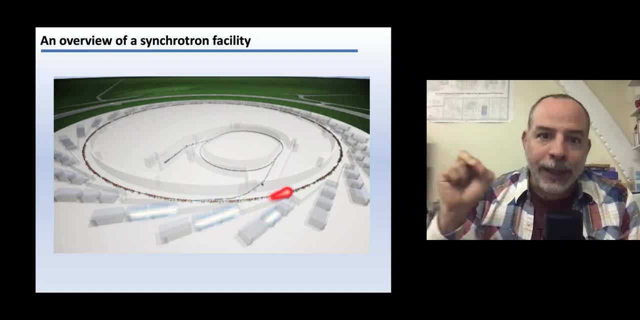 OK, This configuration is very important. First thing, the X-rays. they need to be focused, But, as you can imagine, this is very intense radiation, So health and safety is very important here. You cannot be in the same laboratory where the X-rays are on. 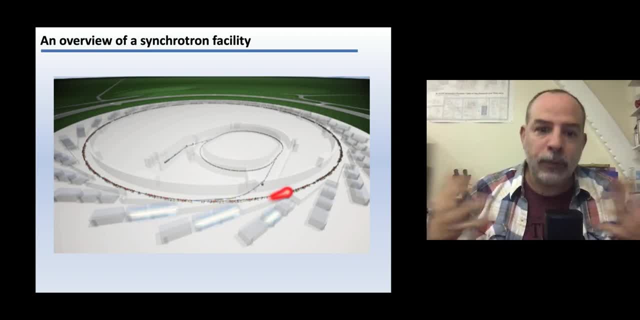 Because this radiation is very intense and harmful for our body. So, therefore, you always need to control the experiments. in this control cabin, You control your experiments remotely. So what happens is that if you want to use a facility like this, what you have to do 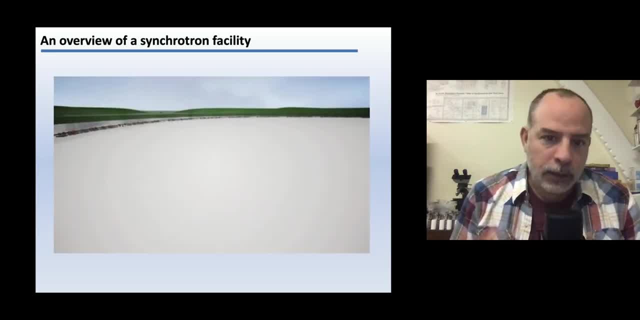 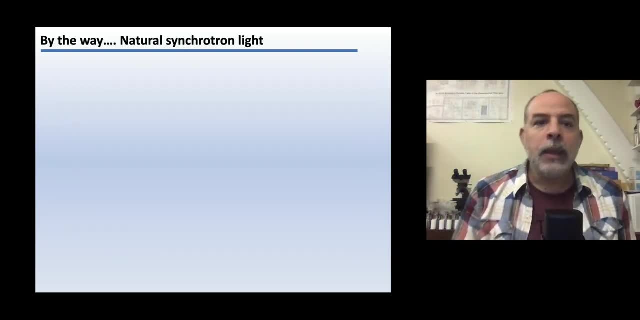 is to write a proposal And then, if your proposal is accepted- this is a competitive process- then you can go to this facility for a few days, OK, OK. So one thing that you probably have heard is that there are natural sources of synchrotron. 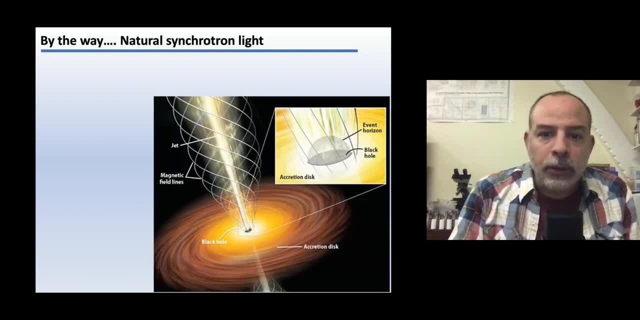 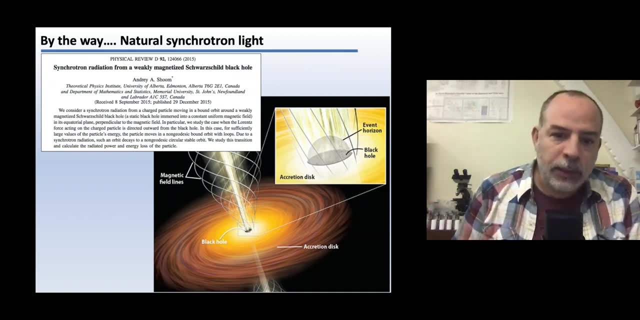 light, And one which is very well known is black holes. OK, Black holes can produce synchrotron light because they have magnetic fields, very strong magnetic fields, and matter moving in circular pathways along these magnetic field lines, And what happens is that, because of this movement of matter, they produce synchrotron radiation. 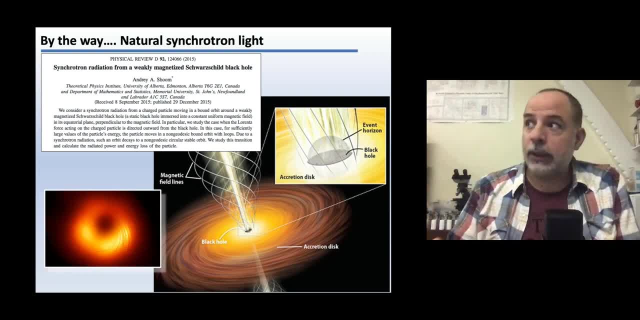 OK, The thing is that this is something which is not natural. OK, This is something that happens in nature. OK, in different places in our galaxy, And this cannot be confused with the synchrotron light which is produced experimentally. 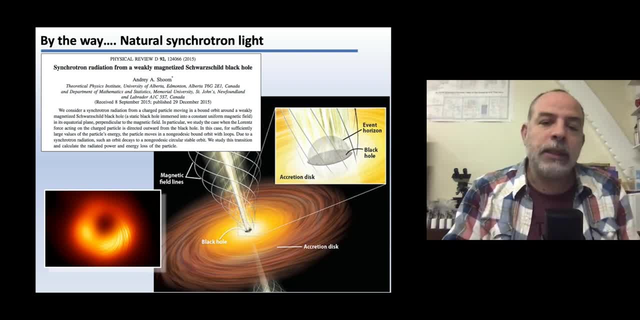 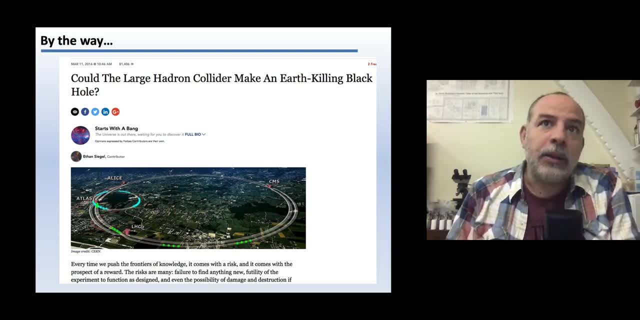 OK, What I mean with this is that you probably have seen news like this: if it is possible that synchrotrons can produce black holes- And I can tell you an answer in a very simple way- The answer is no And no. 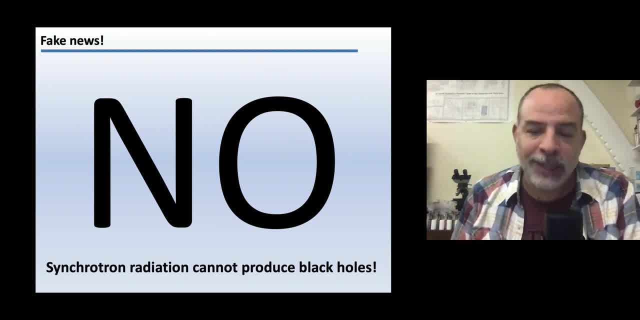 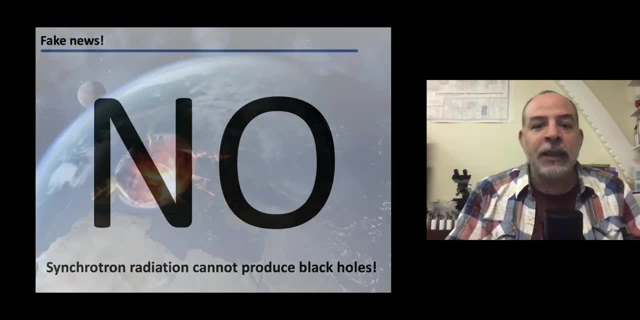 Because a synchrotron radiation cannot produce black holes. OK, Black holes can produce synchrotron radiation, but not the opposite. OK, So therefore, all this news and all this kind of science fiction ideas, you know that a. 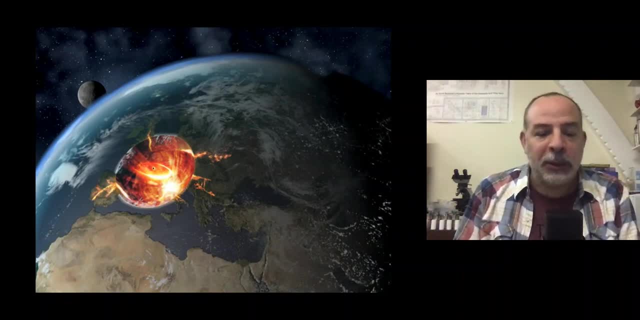 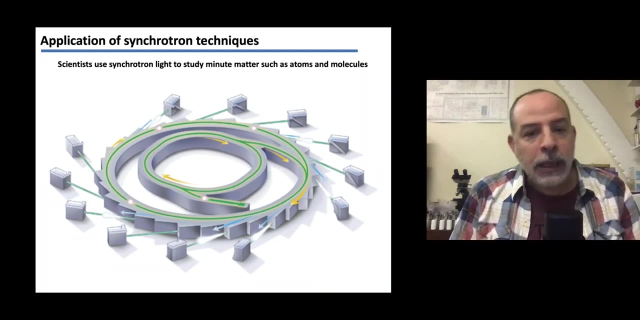 synchrotron could produce black holes and that could be a big problem in our planet. This is not realistic. OK, This is science fiction and not science, All right. So now I'm going to move to the applications of synchrotron techniques. 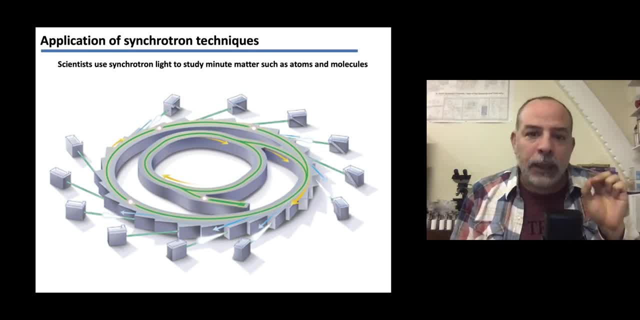 OK, We use synchrotron techniques to understand matter at the atomic level. OK, It's very interesting to understand the structure and nature of matter that way, And this has applications in all the fields of science, And I'm going just to give you some examples. 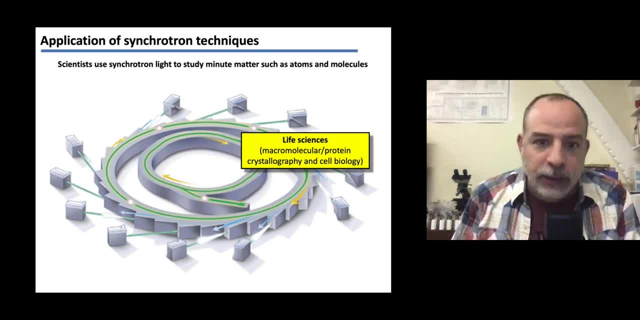 For example, in life science, it's very interesting to use synchrotron radiation to determine the structures of proteins or macromolecules at the atomic scale- OK. Also, there are millions of applications in medicine, OK. For example, from cancer radiation therapy to microbiology, the study of viruses like 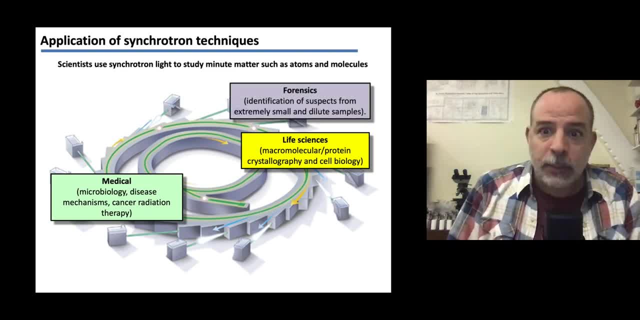 COVID-19.. OK, Also many applications in forensics, because sometimes in forensics there are samples that need to be analyzed and they are very dilute and very small. So synchrotron light has one advantage and it is that the signal to noise is very high. 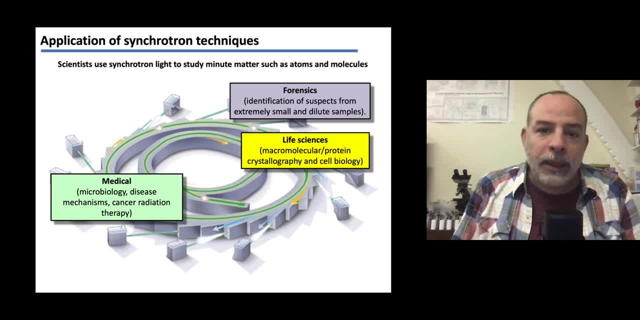 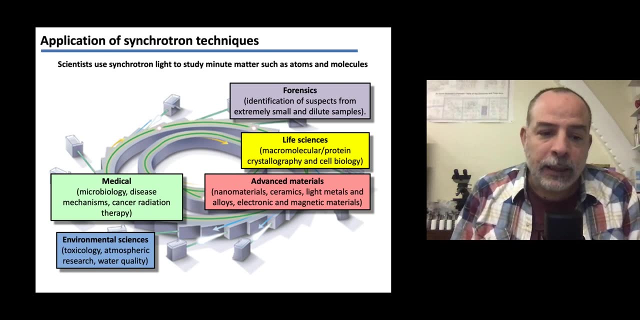 OK, That ratio is very high. Therefore it can be used very successfully in forensics. OK Also for advanced materials, for example for nanomaterials, nanoparticles, ceramics, light metals, electronics. OK Also for environmental science like toxicology, water quality, atmospheric research or for 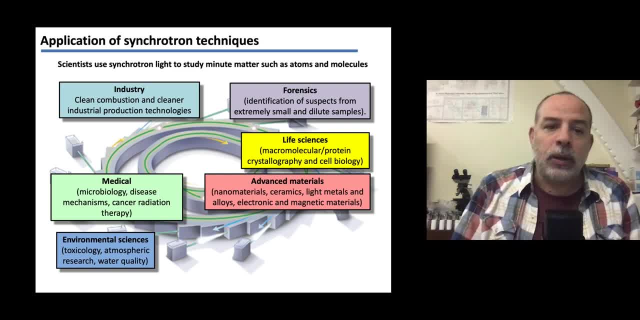 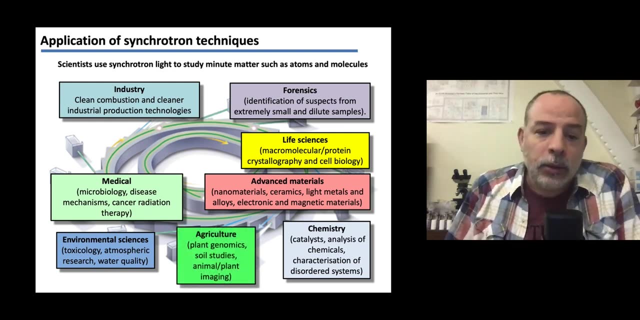 industry, like clean combustion technologies or cleaner industrial production technologies, And, as you can imagine, there are a lot of applications in chemistry, from catalysis to analysis of chemicals or the characterization of amorphous and poorly ordered systems, And in agriculture, for example, like plant imaging, genomics, soil studies. 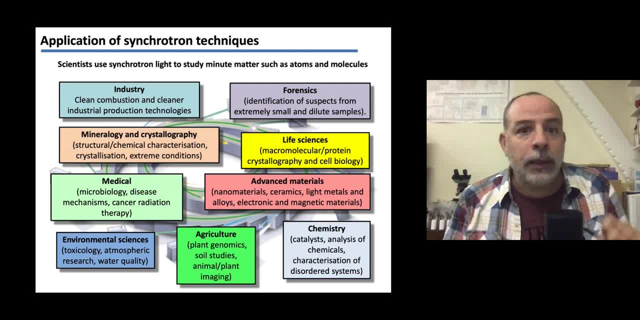 And of course in earth science And in particular in earth science. synchrotron radiation is very interesting in mineralogy and crystallography, In research on crystallization and also research in extreme conditions. I mean high or low temperature pressure. 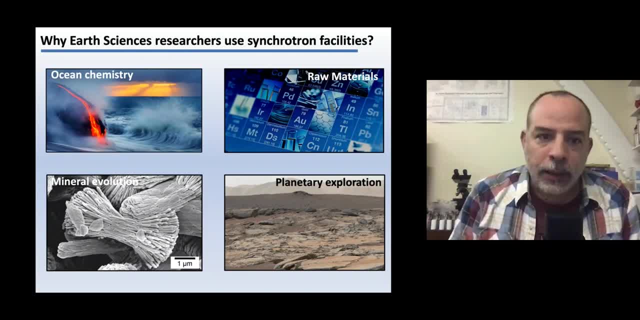 OK, So I'm going to give you some examples in earth science And I'm going to select some examples that can link with many fields of research Like ocean chemistry or mineral evolution, planetary science or raw material, And this field is crystallization. 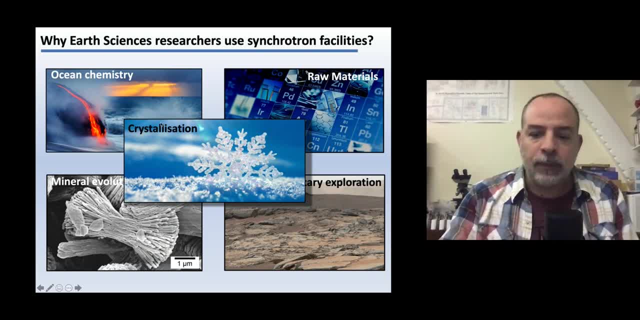 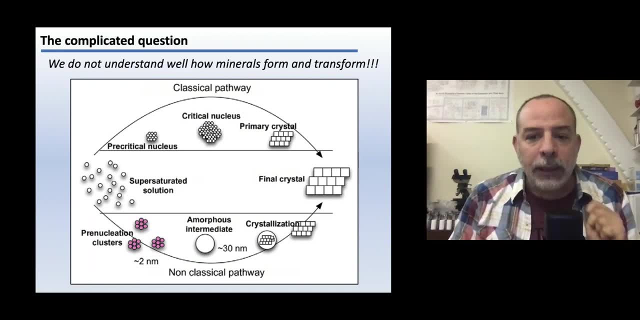 Because crystallization is present in many of these fields. OK, So, in crystallization there is one problem That we don't understand very well: how minerals form and transform, And this happens Because these processes are very fast. We know that from a supersaturated solution we produce crystals. 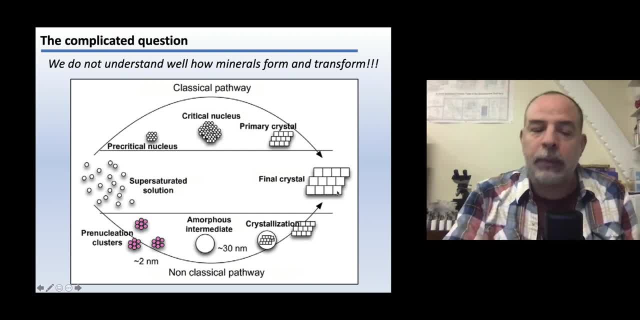 Sometimes this happens by what we call a classical pathway. I mean you crystallize these crystals by forming nuclei which grow OK. Or sometimes it happens by what we call a non-classical pathway. For example, we form pre-nucleation clusters that later form amorphous phases which crystallize. 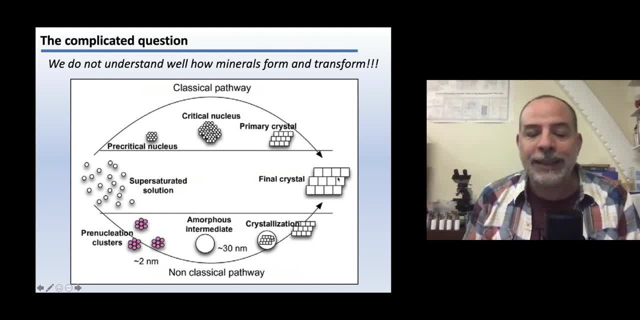 The problem is that these branches- Although this looks very simplistic in this diagram here- These are processes which are extremely fast, They can take place in seconds, tens of seconds- And they are very difficult to follow using conventional techniques. So synchrotron radiation, synchrotron-based techniques, are very useful for this purpose. 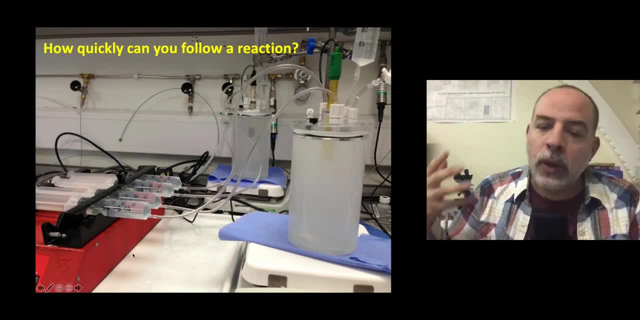 So imagine that you are doing an experiment like this, in which you are crystallizing a solid from a solution- OK, By mixing solutions. So how do you follow the reactions? How do you follow the reactions? here You need to take your solids from the solution. 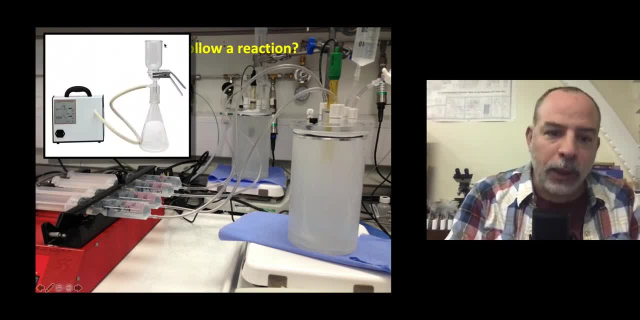 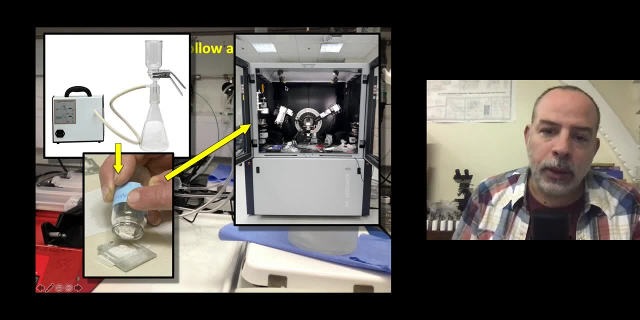 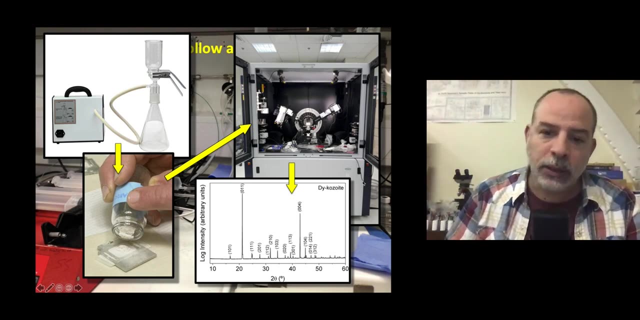 And you can do this by using vacuum filtration. And then you have your powder. You put your powder on a holder, You put this holder with the powder in a powder x-ray diffraction instrument And from here you can obtain structural information. You can identify your phase or phases. 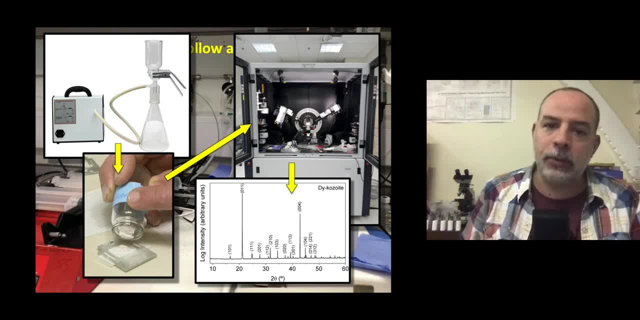 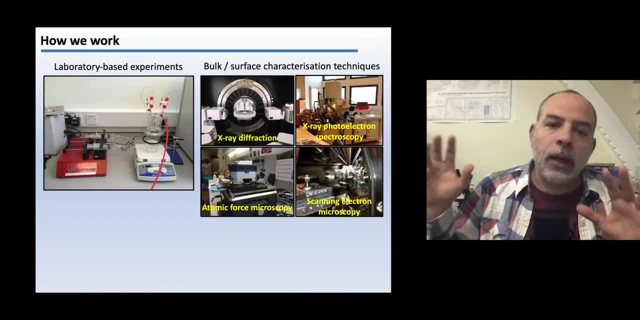 And to do quantification if needed. And then you can go, for example, to the scanning electron microscope To do particles analysis Or size distribution analysis. OK, So synchrotron facilities can make your life easier Because you can obtain much more data. 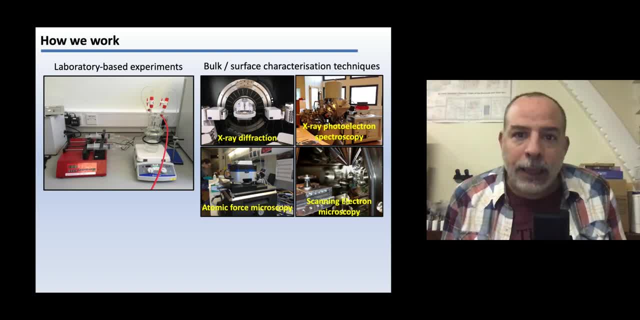 If it happens that your reactions are very quick, you cannot obtain like a thousand samples. That would be very tedious, very complicated, And in fact you can run out of samples Because your experiments have a limited volume. So how do we work when we need to do synchrotron-based studies? 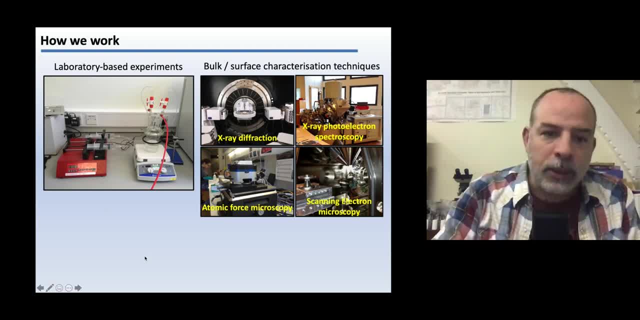 What we do is first we do experiments in the lab And we mix solutions And we use different techniques to characterize the solids, To have a preliminary characterization of the solids, And then we apply for beam time. We apply for beam time at different facilities. 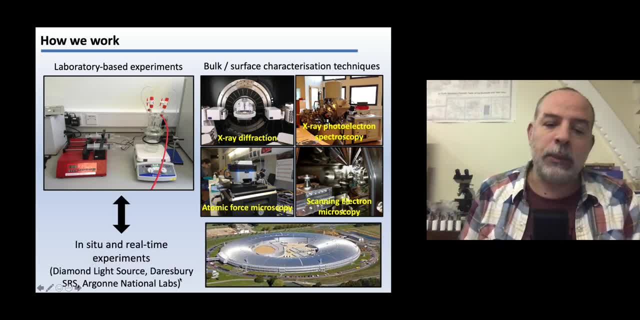 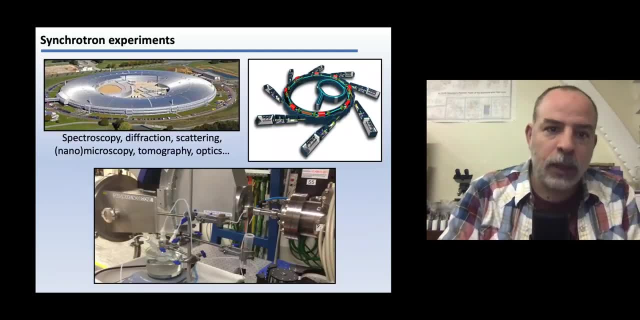 Like at Diamond Light Source, for example, Or Argonne National Laboratories, And if our proposal is successful, then we go there for a few days. OK, Three or four days, All right. There are many different techniques that you can use in synchrotron facilities. 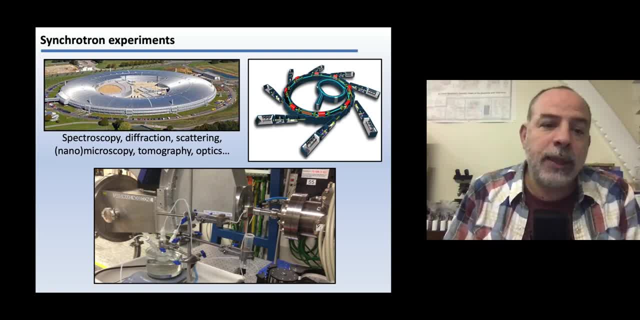 From diffraction, scattering, tomography, optics, spectroscopy, microscopy. But obviously when you write your proposal you have to select which one you want to use, Because it has to provide the data you want for your experiments. OK, 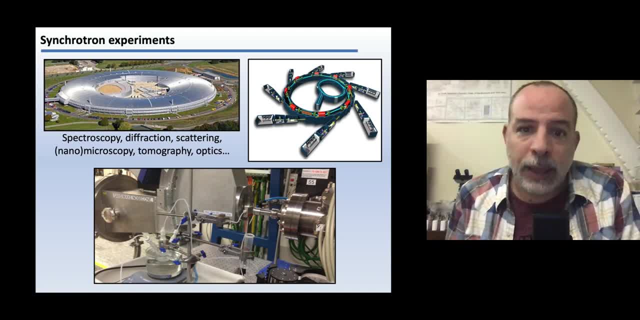 So we select one. For example, in our case, we do small-angle and wide-angle stray scattering, And what we have to ensure is that we can run our experiments in this facility. OK, For example, here you have one experiment in which we are mixing solutions. 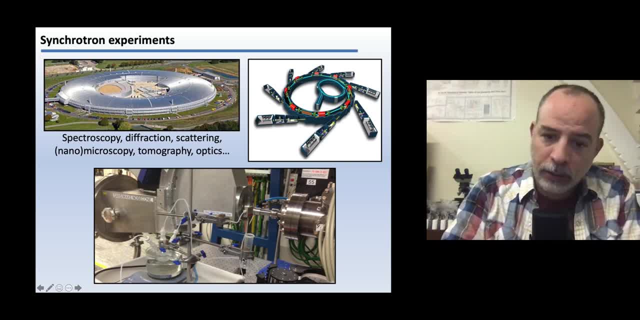 And what happens is that the solution goes through this tube here And through this capillary, And through this capillary And goes back And the X-rays, the synchrotron X-rays, go through the capillary. So we can probe what is happening in our solution, with our particles, as long as we want. 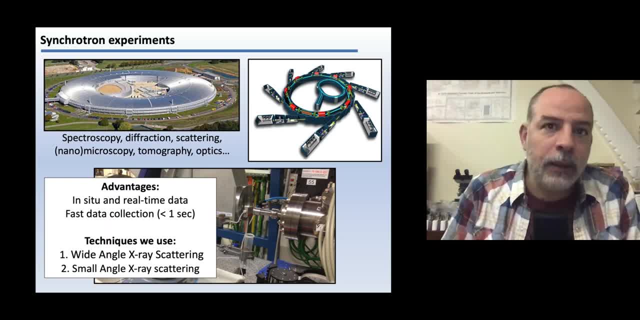 OK, We can collect data in time intervals of less than one second. We can have in situ and real-time data, And that way we can obtain very useful kinetic and mechanistic data. OK, That's the approach. So overall, what we do is: 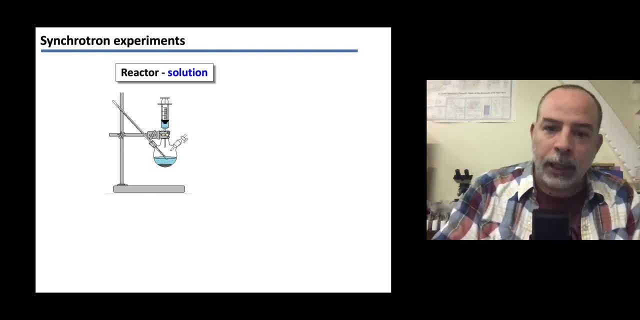 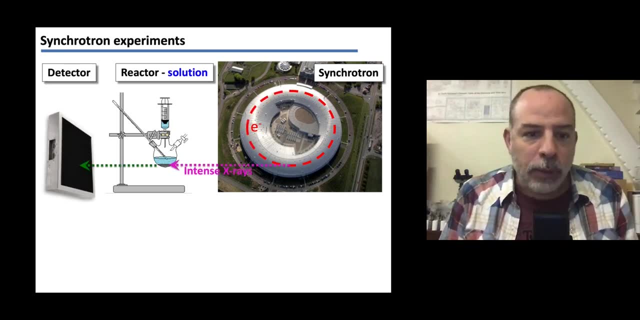 We have our experiments in the synchrotron, And the synchrotron, by using electron, is producing X-rays that will go through our sample. This data will be collected with one or several detectors And from here we obtain two main pieces of data. 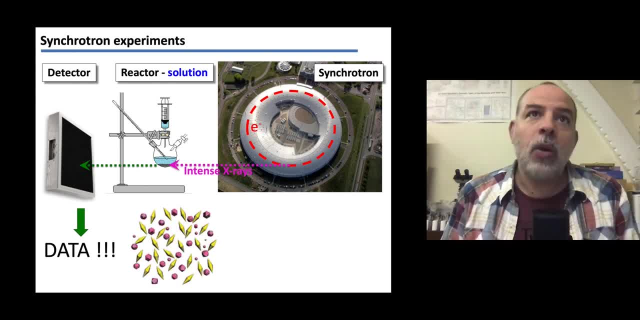 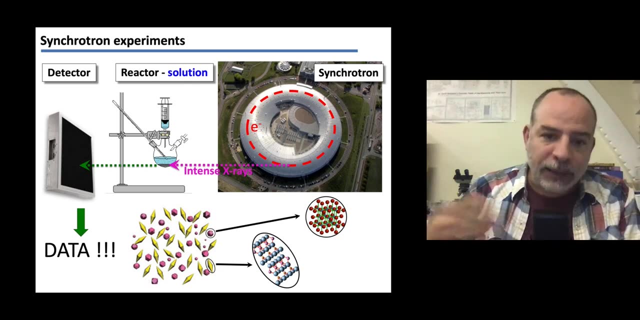 First thing is particle size distribution. We can infer what are the particle size distributions as a function of time in our experiment. Second thing is particle identification. What I mean with this is that we can identify which particle size distribution we want. We can identify which minerals we have in our experiment as a function of time. 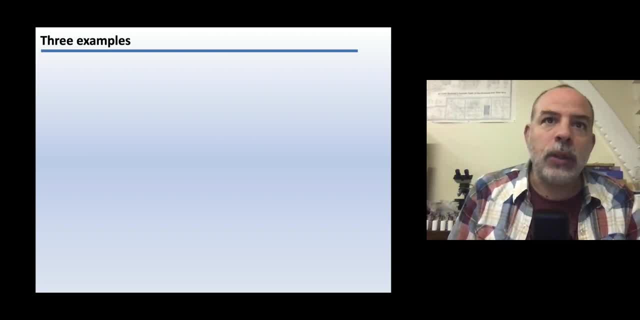 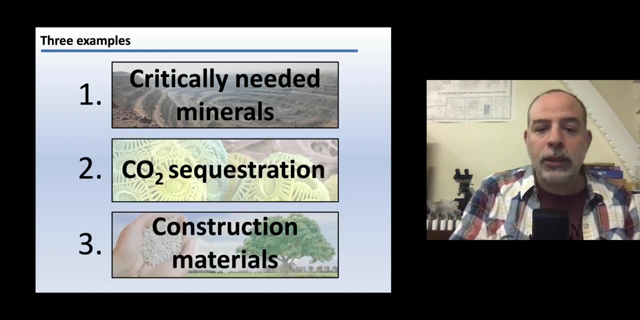 OK, And I'm going to show you now three examples to demonstrate how useful these techniques can be for us. The three examples will go from easy to more complex: synchrotron data, And I'm going to focus on critically needed minerals, then on CO2 sequestration, and also on construction materials. 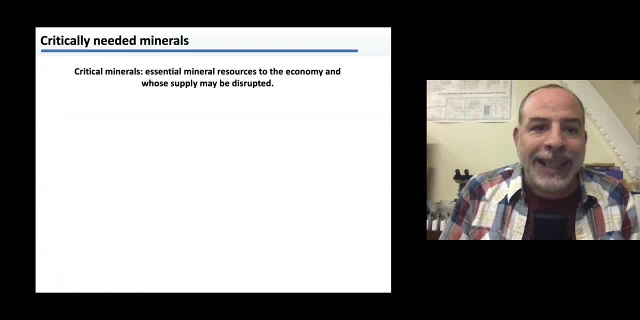 So I'm going to start with the critically needed minerals. OK, Critical needed minerals are these ones which are essential for the economy, And the problem is that the supply may be disrupted, And typical examples are the elements that are used to build smartphones or computers. 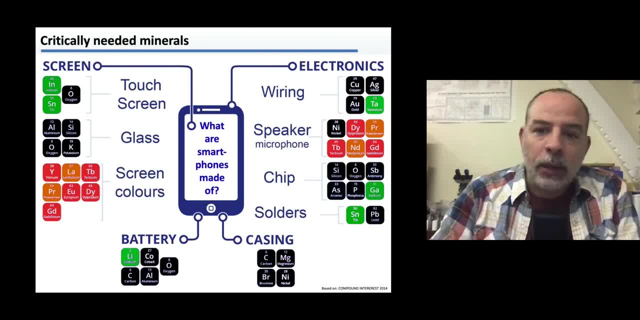 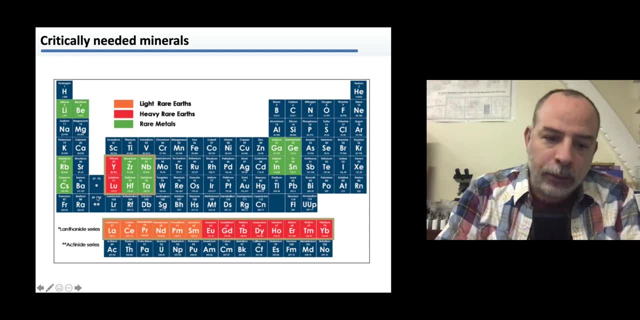 Many of the elements that we use to build smartphones are the rare elements here in red or other elements, which are gallium, tin, indium, lithium, OK. These elements are very interesting for modern technologies and carbon clean technology, For example. the rare elements are here at the bottom: the light rare elements and the heavy rare elements. 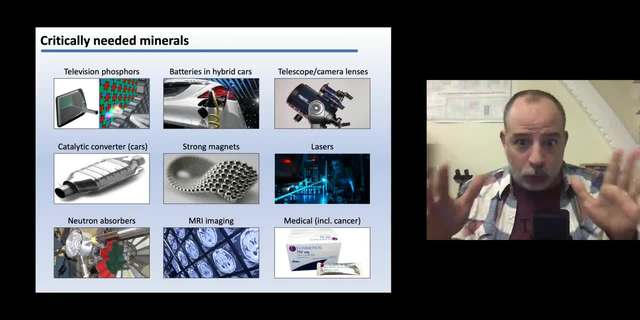 OK, These rare elements, for example- and I'm going to focus on these rare elements- they are used for many different types of technologies, To produce magnets, for catalysis, for lasers, for lenses, for batteries, for many more things. 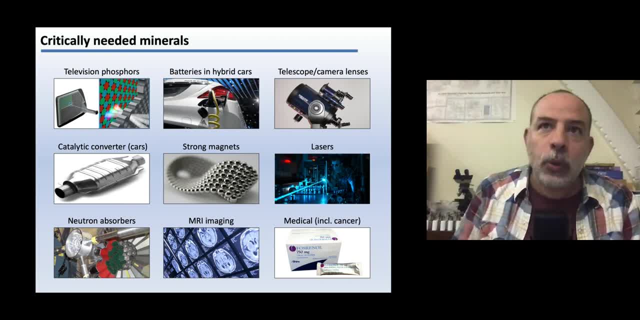 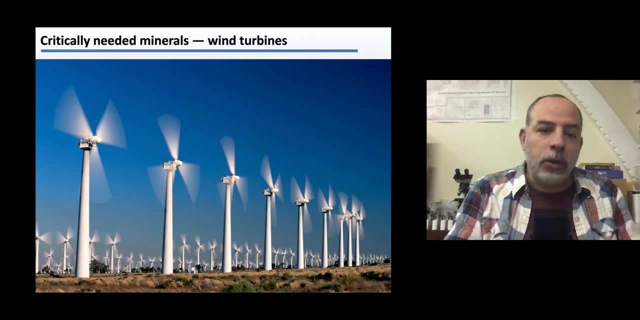 They have medical applications. they have industrial applications a lot. OK, They are essential every day And the economy depends on their availability, On the availability of these rare elements for industry. For example, in Ireland we use wind turbines to obtain energy. 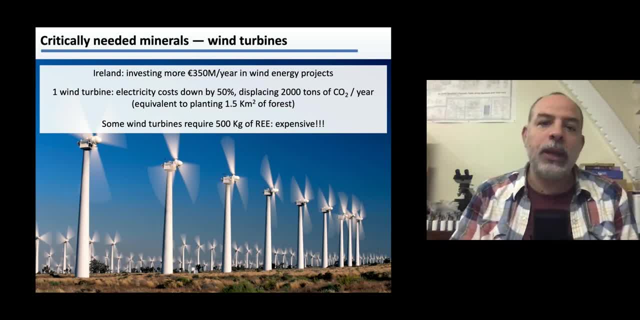 And every year Ireland invests more than 350 million euros in wind energy, Because one turbine like this can decrease electricity in 50% and can displace a good number of tons of CO2.. The problem is that these wind turbines they require half a ton of rare earth elements sometimes. 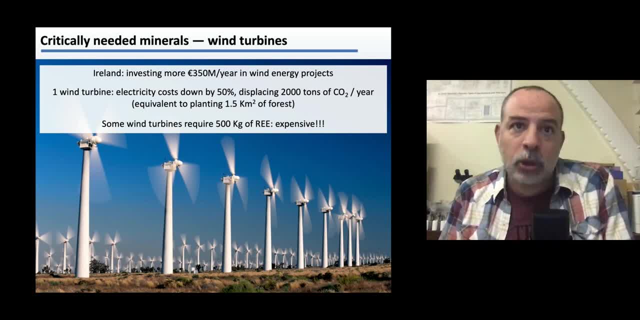 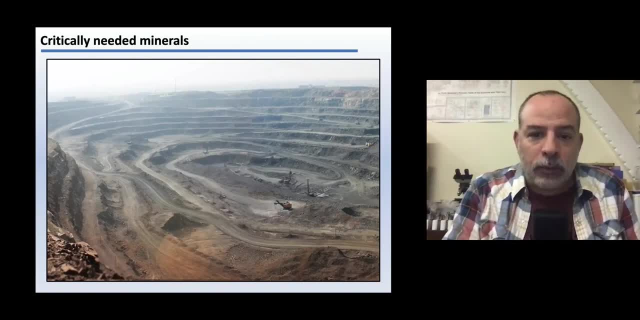 So they are very expensive, And they are expensive mostly because of these rare earth elements. This is a complicated market. Rare earth elements are obtained from rocks, In particular from some deposits, which are carbonate deposits mostly, And the rocks could look like this: 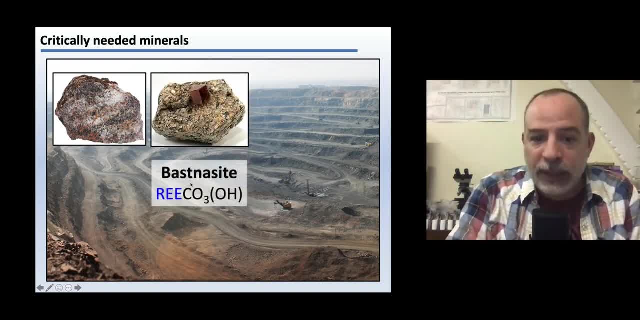 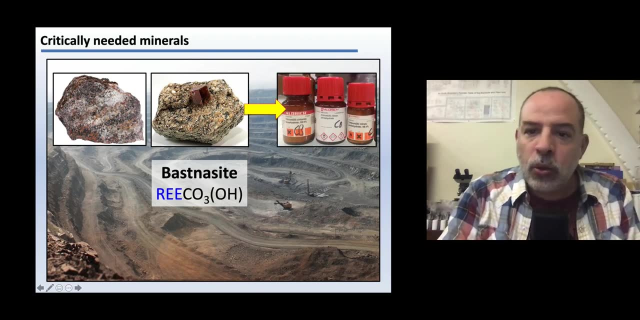 If you are lucky, you can have a bigger crystal of this phase named bastazite, which is a rare earth carbonate, And what happens here is that this bastazite contains the rare earth elements that we use for industrial applications, But we need to go from something like this to something like that. 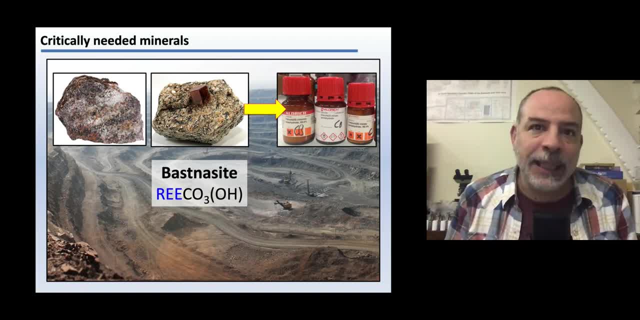 Because we need pure rare earth elements, We need high purity, And each industrial application requires essentially one or maximum two rare earth elements- Not all of them, And the problem is that ideally, we would like to have crystals like this that contain, for example, one rare earth element. 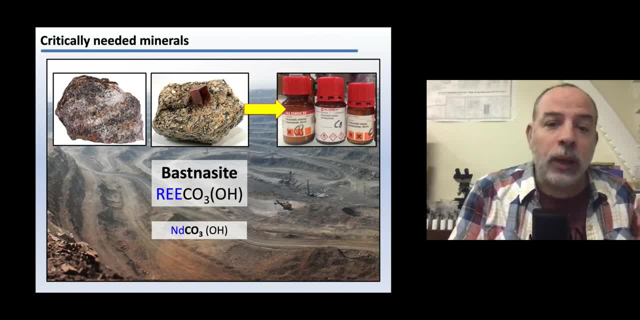 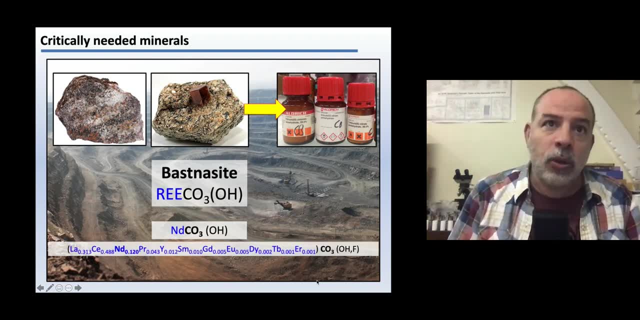 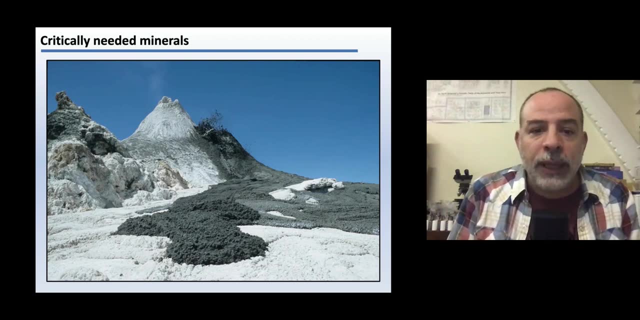 But nature is more complicated than that. So in these crystals, in these bastazite crystals, what happens is that we find all the rare earth elements in different proportions. So separation is very complicated And purification is even more So. also, there are not many active deposits that concentrate rare earth elements. 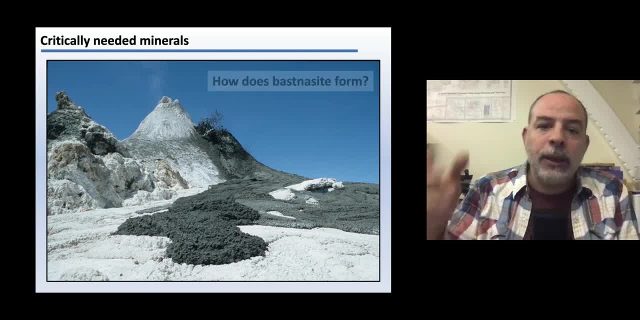 This is one in Tanzania. It's a carbonate-type deposit And the problem is that we don't know how the minerals you have seen before forms. That mineral is named bastazite And it is one of the three minerals which are the main sources of rare earth elements for industry. 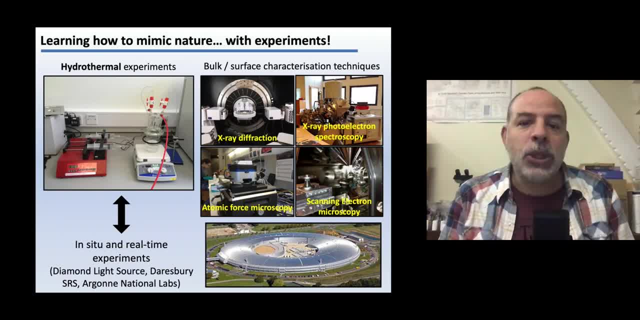 So, as I told you, what we do is to try to mimic what happens in nature by using experiments. So we combine first offline experiments, laboratory experiments, with synchrotron experiments, in this case to understand how a mineral like bastazite forms. 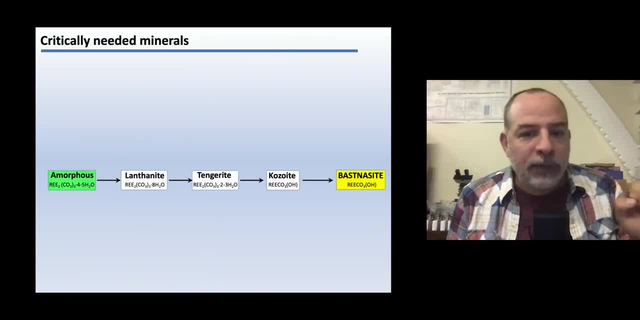 So OK. So we have seen that bastazite forms from an amorphous phase And we have synchrotron data showing us that this transformation from amorphous to bastazite takes place via different polymorphs. They are named: lanthanide, tengeride, kosoide. 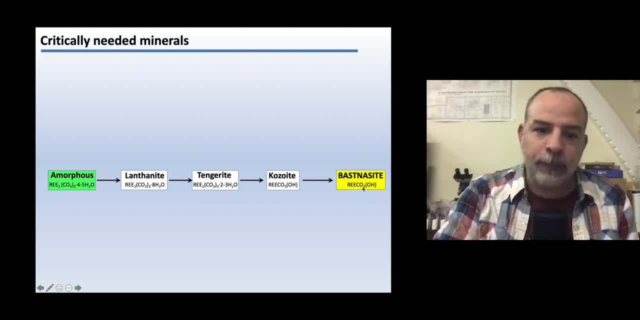 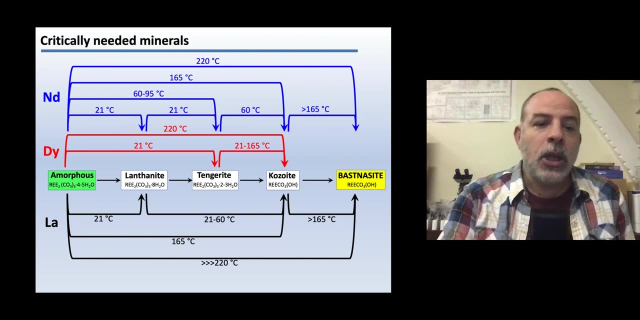 And these ones slowly transform into bastazite. This transformation depends on the rare earth element involved. The kinetics and the temperatures required depend on the rare earth element, And therefore this is a very complex system to work. So one thing that we have been trying to understand is what happens at the early stages. 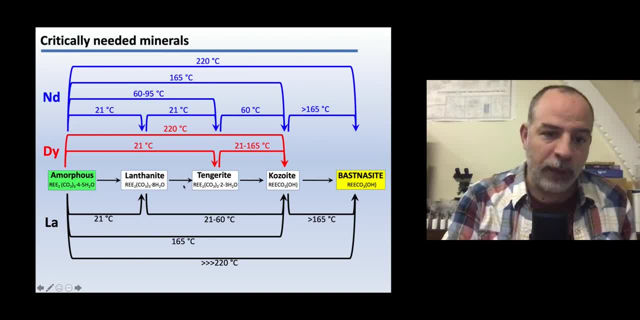 When we form an amorphous phase and then transform to the first polymer, lanthanide, Because we want to know if something else is forming here. So I am going to show you one simple experiment using synchrotron-based diffraction. 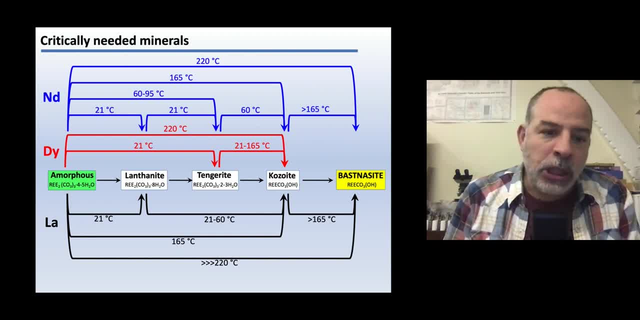 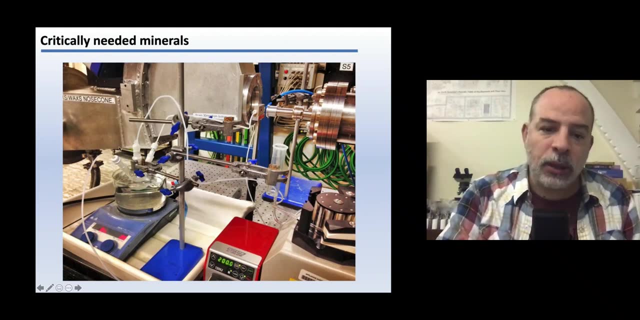 in which you are going to see the transformation from amorphous phase to this mineral named lanthanide, Because we want to know what is happening here. So what we do is we produce this lanthanide here by mixing solutions, Then the solution goes through this tubing and then through this capillary here. 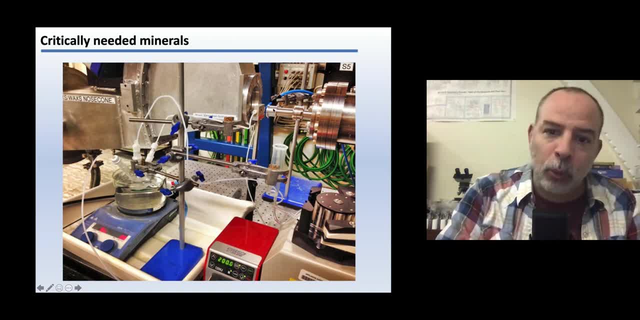 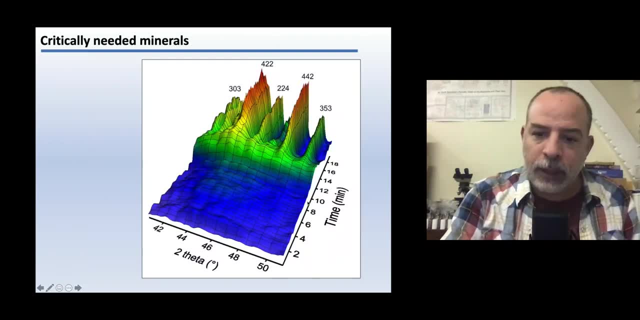 And the x-rays, the synchrotron x-rays, are probing the volume of water plus particles in there. So what do we see That we have here? time in minutes, Ok, And this is something named 2θ, If you don't know what is this. this is coming from x-ray diffraction. 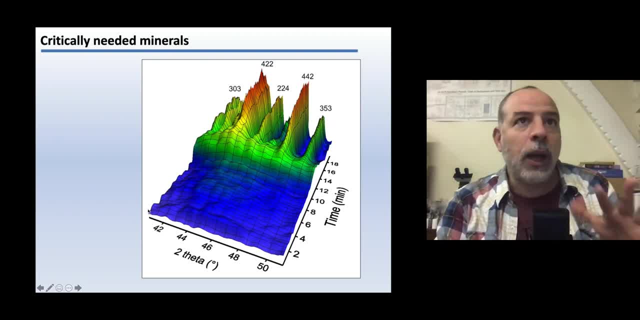 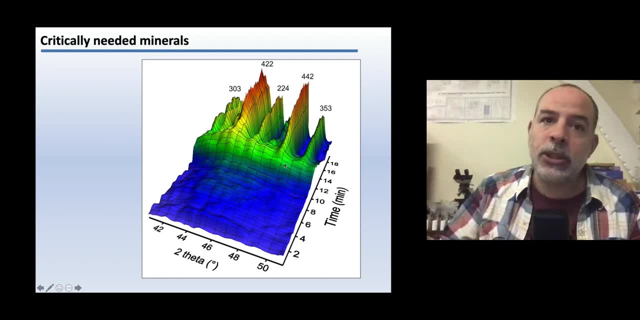 So this is an angle, And if you have never done x-ray diffraction, I will tell you two clues to understand what we obtain here. If you have no peaks, that means that your material is non-crystalline, It is amorphous. 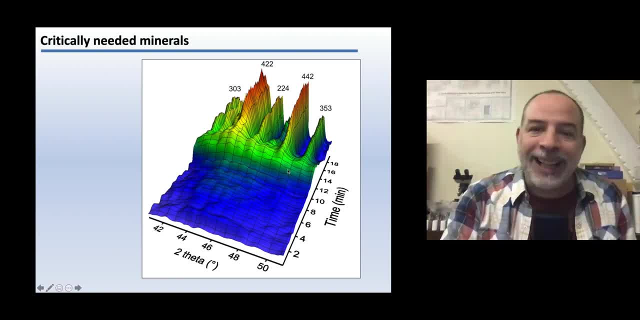 When you have peaks. that means that you have a crystalline material, a mineral, And the position of these peaks will tell you what mineral you have. You can identify your mineral by knowing the specific position of the mineral, The position of the different peaks. 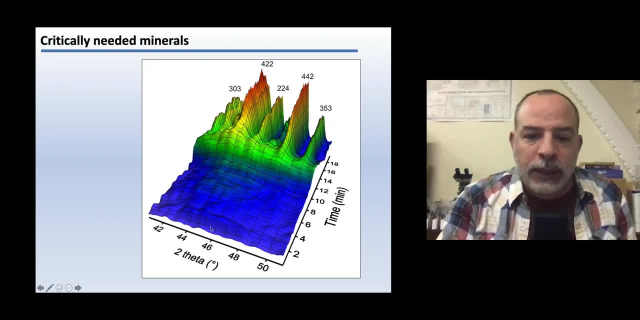 They are named Bragg peaks. Ok, So here, what we see is that at the very early stages of the reaction, we have an amorphous phase that then transforms into something crystalline, And this is what we have been following by using also conventional techniques. 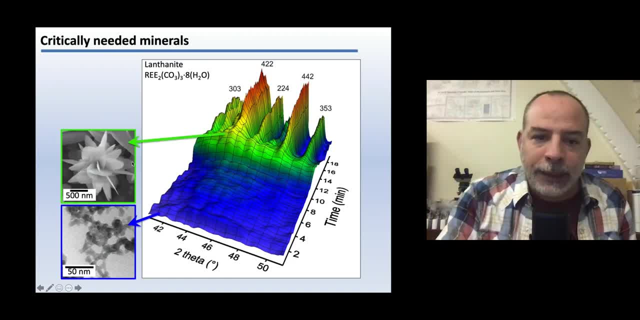 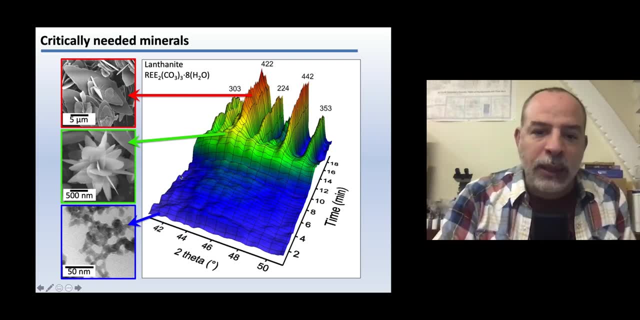 So we have at the beginning an amorphous phase that then starts to crystallize and transforms into a fully developed crystalline material. Ok, So in this case we didn't see anything else forming here. Sometimes in this kind of reaction you can have metastable phases that can be stable for only a few minutes. 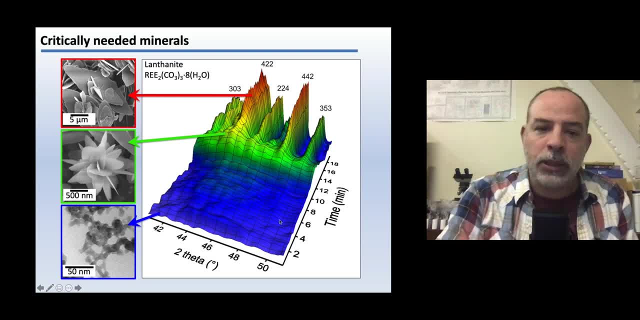 In these cases it didn't happen. So you see here the full transformation of an amorphous phase into lanthanide in a matter of a few minutes. Ok, This is the first stage of crystallization of basaltite. Ok. 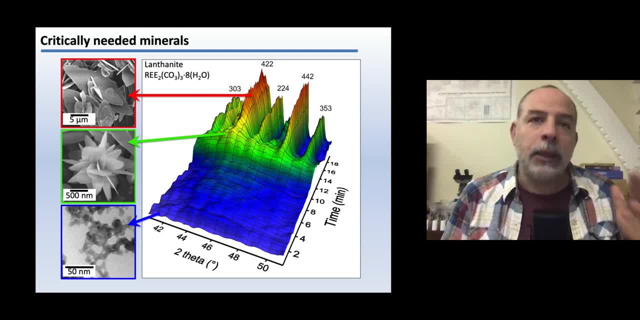 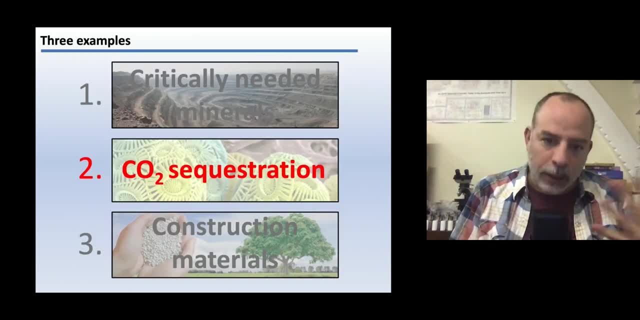 We have followed these reactions in situ and in real time, at different temperatures and with different relative elements. Now I am going to give you now more synchrotron data, So I am going to show you how this picture can be more complex. 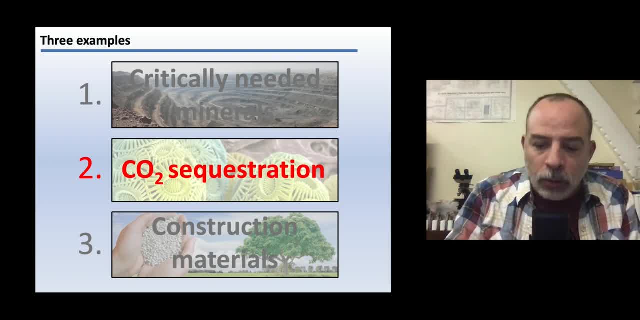 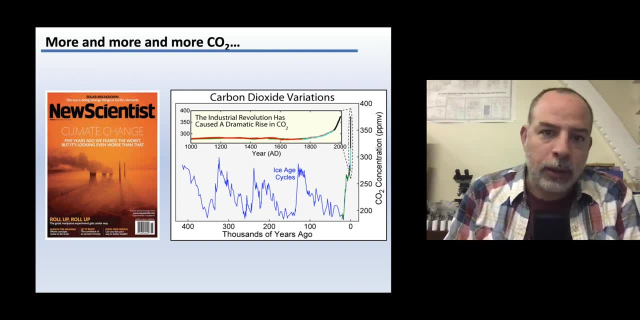 And I am going to focus on CO2 sequestration. As you know, there are many projects today to try to tackle the real dramatic situation with the increase of CO2 in our atmosphere. So there are many projects ongoing in many different places, but perhaps the most famous one is taking place in Iceland. 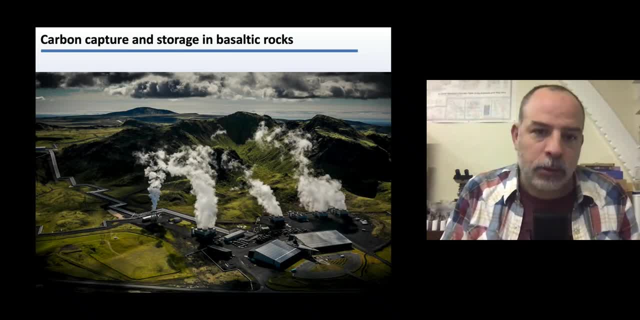 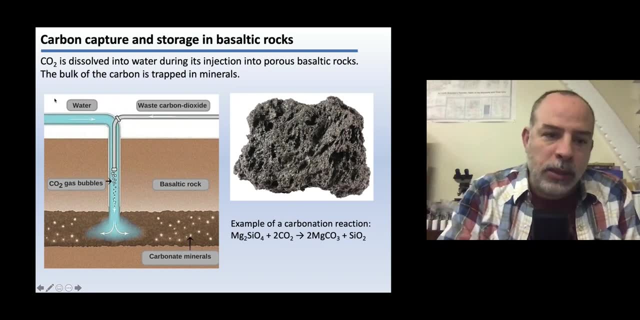 Where carbon is being captured, Being captured in basaltic rocks in a place close to a power plant. Ok, And here what is being done is to inject water and CO2.. They are mixed together, forming something like a soda, And this soda-type water is interacting with basaltic rocks. 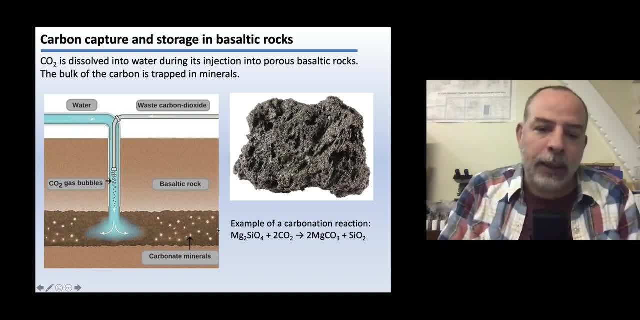 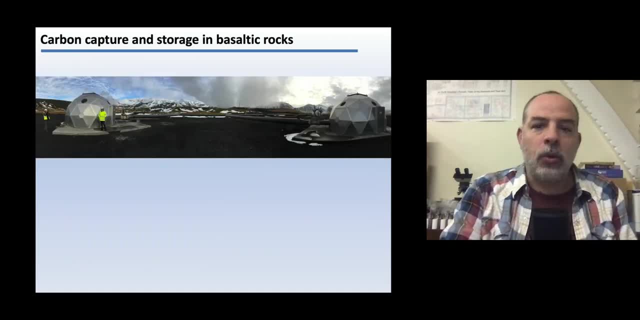 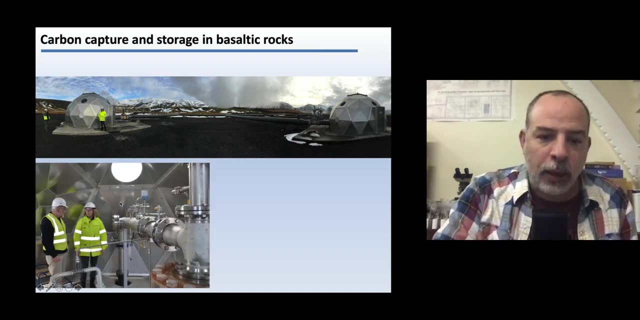 And these basaltic rocks are providing elements like magnesium, calcium and iron And triggering the crystallization of carbonate minerals. Ok, So this is the place. Now it looks like a science fiction landscape, And what you see here is how the CO2 and water is being injected. 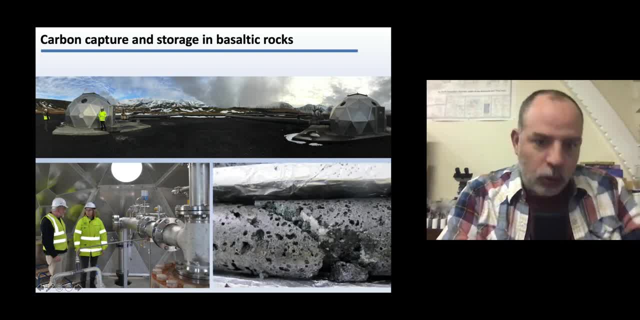 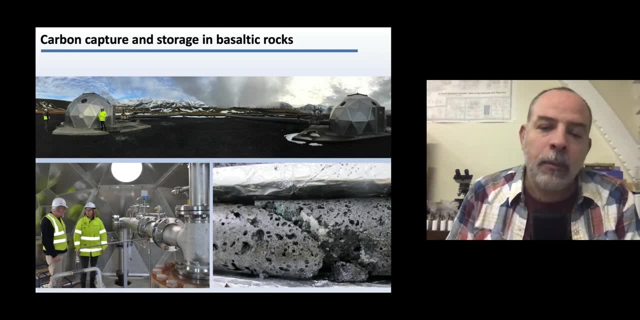 And what happens here is that when you take samples, cores of the material, with time, you see this white precipitate. This is the carbonates. This is carbonates forming via this interaction of basaltic rocks and soda-type water. Ok, 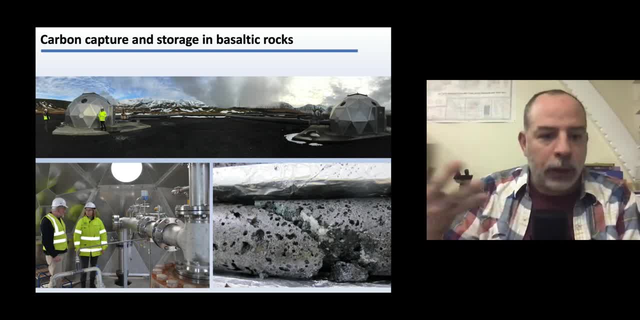 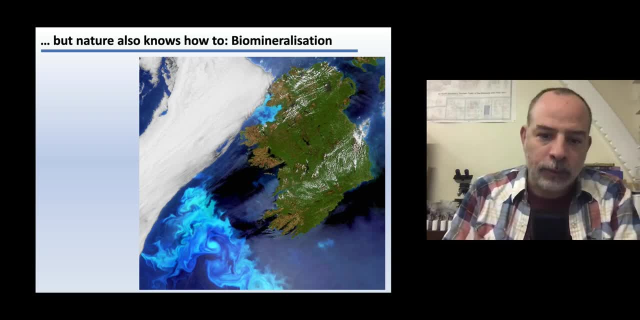 Water with CO2.. With dissolved CO2.. All right, We know that this can be done, But we also know that carbon sequestration- Carbon sequestration- is also happening in nature, And there are living organisms which are producing calcium carbonate by forming skeletons and cells. 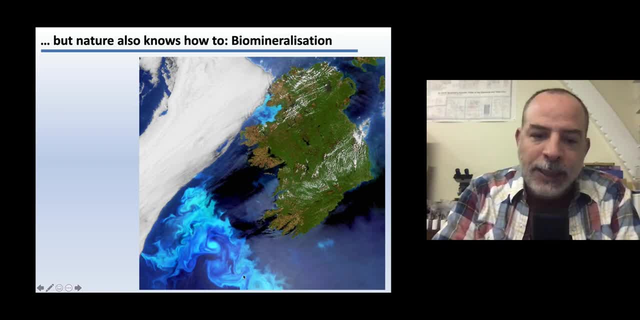 For example, you see here one picture where you can see this blue area. This blue area is: This is not a cloud, This is an accumulation of different algae. They are named coccoliths And they happen to scatter the light. 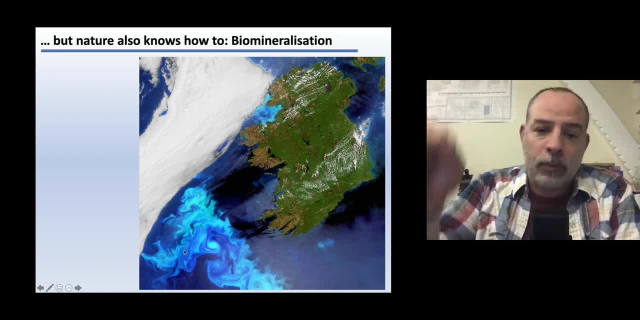 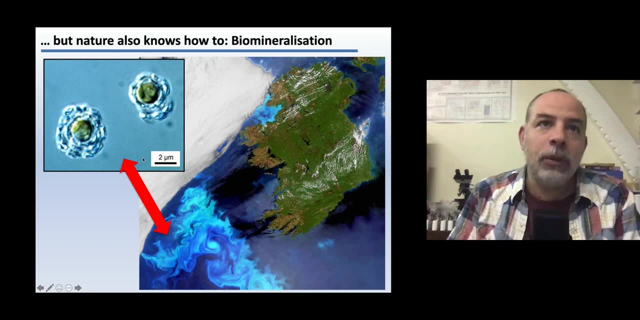 So you can see this. You could see this from a satellite, And this is light scattered by these coccoliths. These coccoliths are algae, And what happens with these coccoliths is that they are able to produce skeletons, cells of calcium carbonate. 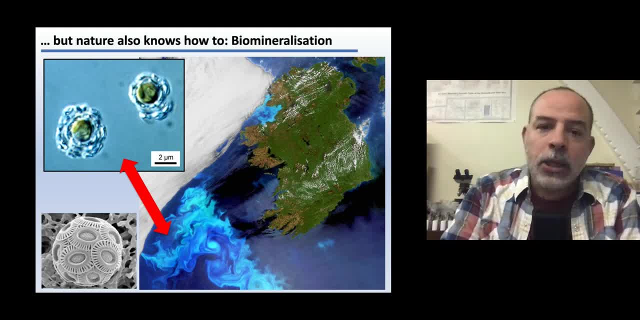 Of calcite. Ok, They look like that. I'm sure you have seen many of them. So the problem is that here we don't know how this calcite is being produced inside these cells. And why is that? First, because they are very small. 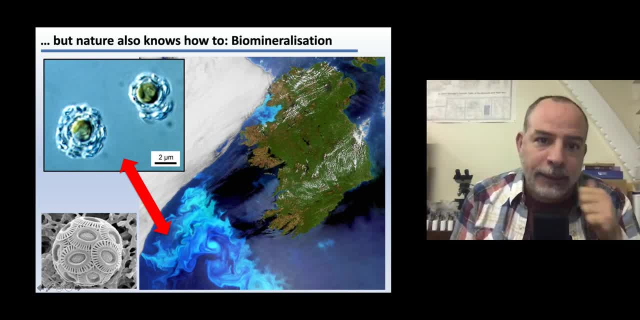 You see the sizes here. This is less than 2 micrometers. Second, because there are many organics here and there is life involved. So there is likely high supersaturation processes taking place here which are producing an amorphous phase which is crystallizing later on. 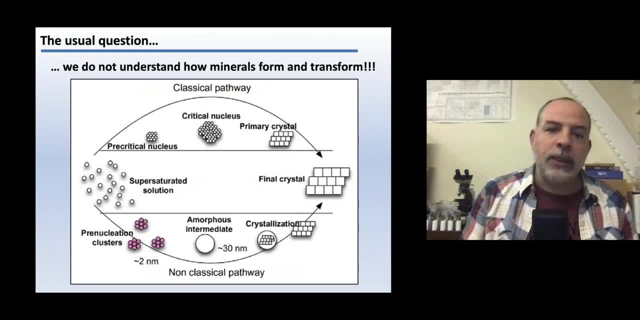 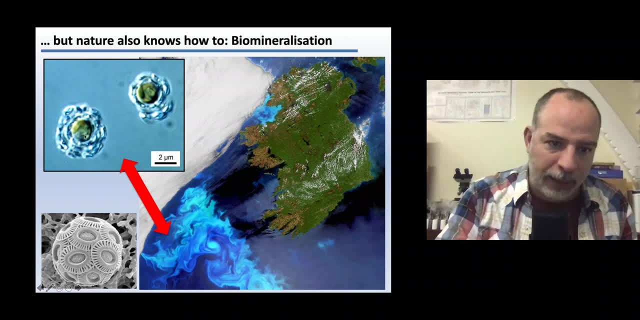 So is it possible to mimic these experiments in the laboratory? It is, And this is what we try to do. We try to understand what happens when we have a supersaturated solution, similar to what may happen inside these cells, And how crystals can form. 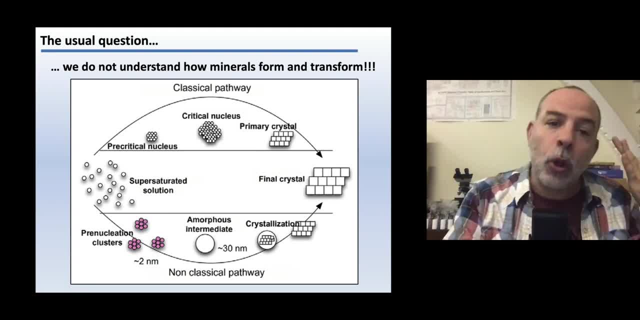 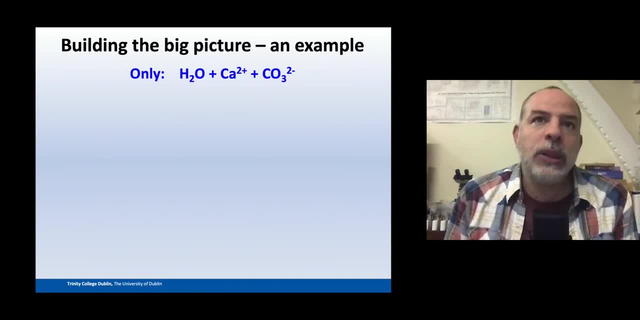 Ok, And I'm going to show you some examples of crystallization of calcium and magnesium carbonates. Ok, First I'm going to try to build this big picture by showing you the many different crystallization pathways that can happen when we only have calcium carbonate and, of course, water. 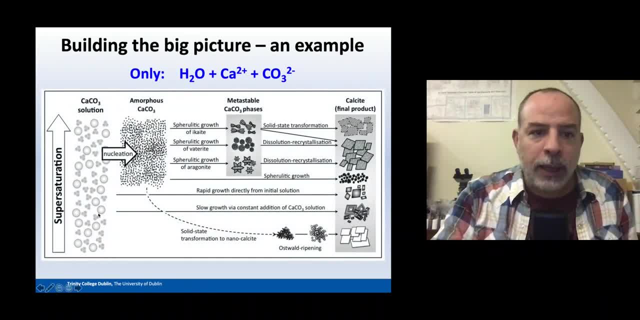 Ok, So here you have a calcium carbonate solution, And this is showing you this solution as a function of supersaturation- Low supersaturation, high supersaturation- And there are many different crystallization pathways taking place depending on supersaturation. 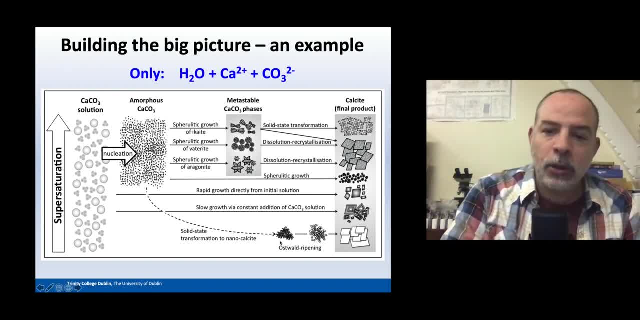 Sometimes you can directly form calcite from solution, Sometimes you form calcite via an amorphous phase, And sometimes you form calcite via an amorphous phase And some metastable intermediate phases that form quickly by spheroid growth and transform into calcite via dissolution and recrystallization. 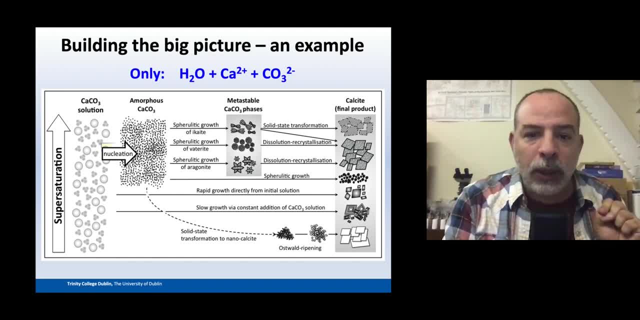 Ok, This is a very well known picture, And what I'm going to show you is what happens following this branch. here, Ok, The crystallization from amorphous phase to calcite via batterite. And also here, decrystallization of calcite directly from an amorphous phase. 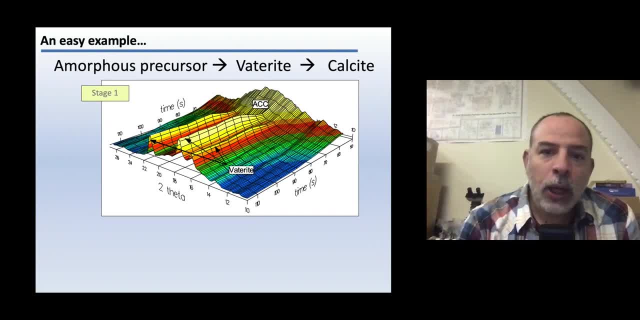 Ok. So this is a perfect example to show you how useful synchrotron radiation can be to follow experiments in situ in real time, Because what you see here is something that took place in less than a minute, So this is 50 seconds. 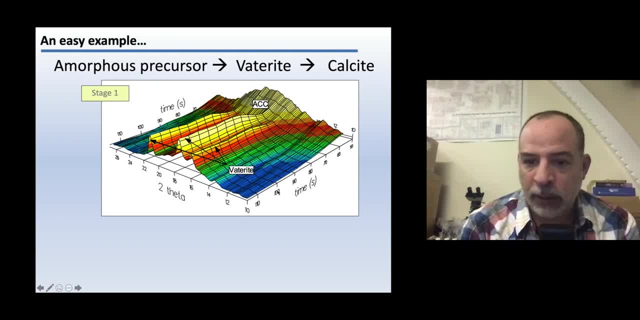 This is less than two minutes. Ok, So one minute of time interval And this is Suthitha. So these peaks are indicating us what mineral phase we have. So at the beginning we have an amorphous phase, an amorphous calcium carbonate. 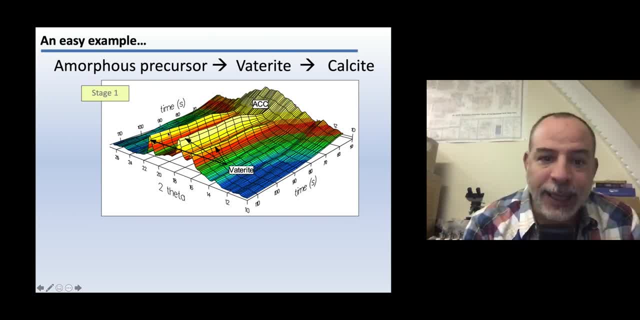 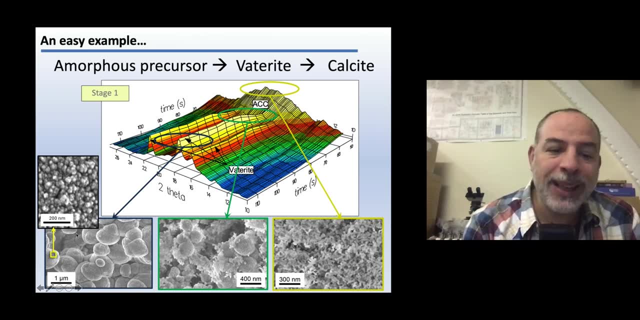 And it's quickly crystallizing into batterite. This crystallization is taking place via one process named spheroid growth, In which the amorphous phase breaks down and batterite quickly forms from this amorphous phase. And these are not single crystals. 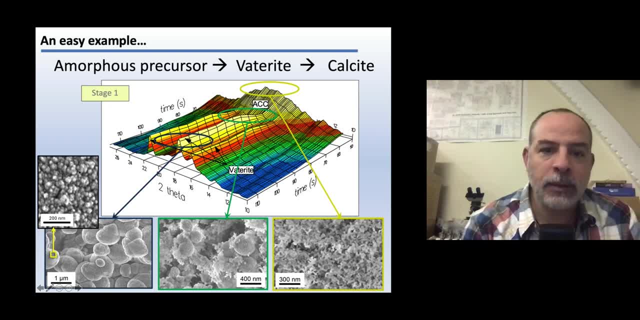 These are aggregates that contain many nanocrystals. Ok, So this is extremely fast crystallization of batterite, And batterite then transforms into calcite. The crystallization of calcite- The crystallization of calcite, takes place much slower compared to batterite. 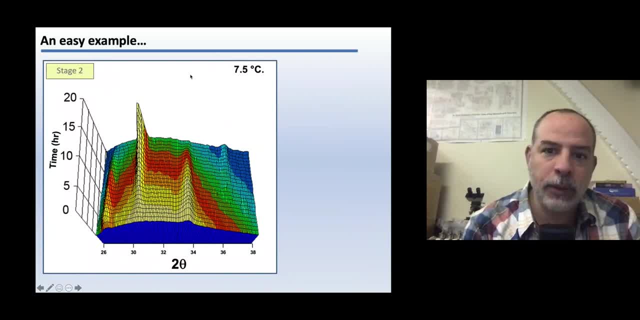 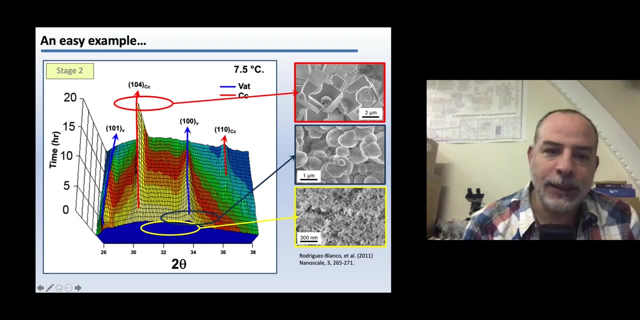 So you can see that here. This is 20 hours. This happened at 7 degrees C And what you see here is the peaks of batterite decreasing and the peaks of calcite increasing. So what you are seeing here is the slow dissolution of batterite and crystallization of calcite. 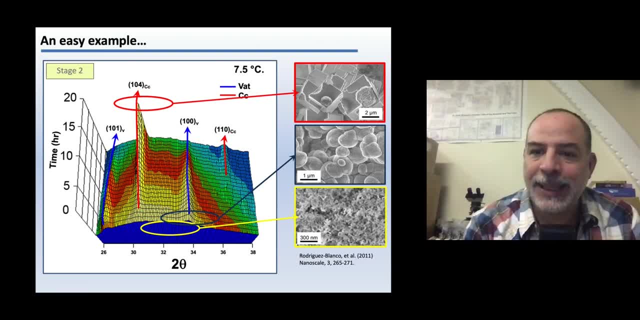 That requires several hours of time. Ok, In this case, at the end we have single crystals. This is a completely different process. This is dissolution, recrystallization- Ok, So this is a different way of showing you the same data. 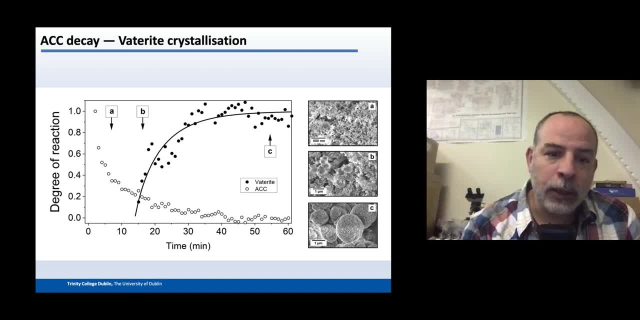 So, in order to show you these 3D plots, we can present the data using these graphs in which you have time And you have here the degree of reaction. Ok, Degree of reaction. If you don't know what is that, You only have to assume that this is like 100% of material phases and this is 0%. 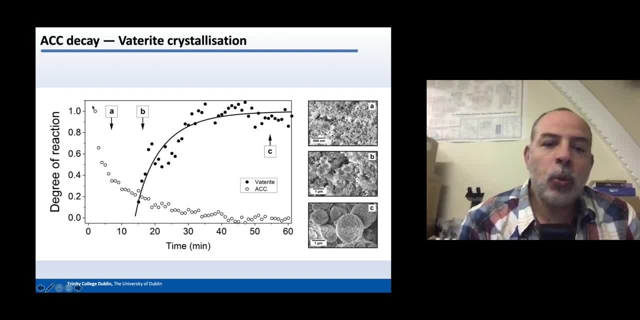 This is like the abundance of each phase. So what do we have here? We have amorphous station carbonate. These are the white dots which are breaking down and quickly batterite is forming Ok, And this happened at low temperatures, about 7.5 degrees C. 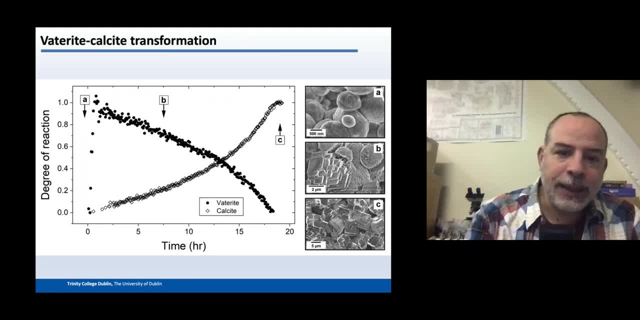 And then, after this process, what we see is that calcite was growing from batterite. But here you see, the time is different. This is 20 hours, And this was a very long experiment in which batterite was slowly decaying, dissolving. 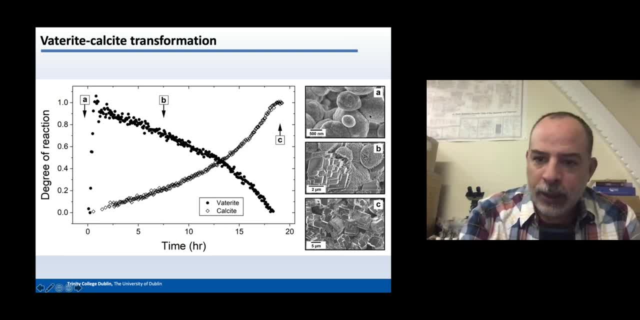 And calcite was decreasing And calcite was slowly growing. Ok, This is what you see in the pictures. These spherulites of batterite are slowly dissolving And calcite is forming via dissolution and recrystallization. 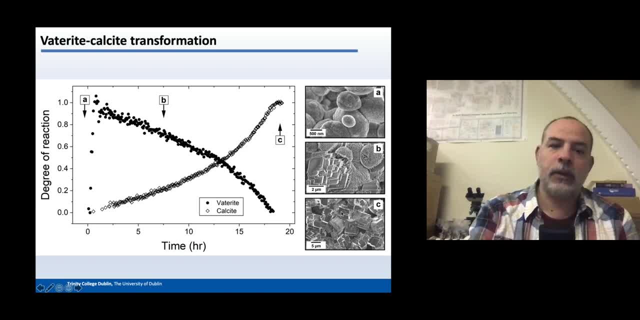 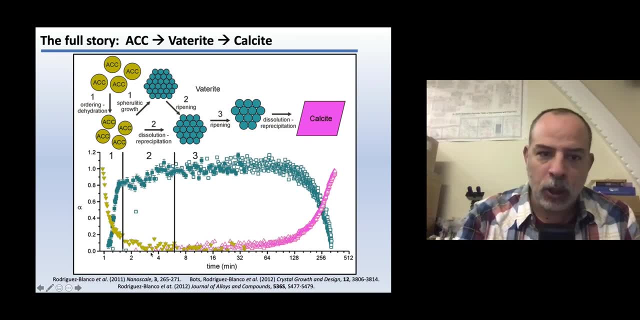 And at the end you have finally only calcite. Ok, So if you put all this together, you could have a picture like this, In which you have a quick decay of the amorphous station carbonate, Extremely quick growth of batterite via spherulitic growth. 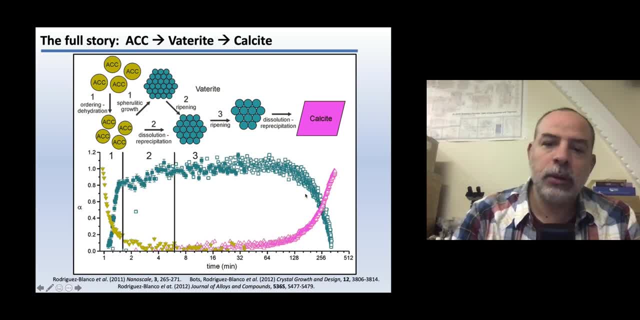 And then a slow decay, dissolution of batterite and crystallization of calcite. This is the full picture, But it would be impossible to obtain this picture without using synchrotron-based techniques, Because you can see here time, And this time is not linear. 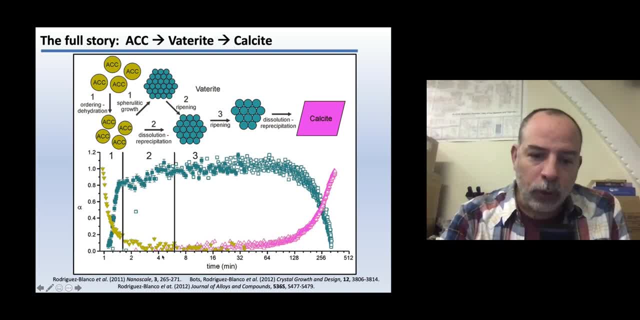 Ok, It's logarithmic, And you see here 1,, 2,, 4,, 8 minutes. So in 10 minutes more or less half of the reaction has happened. Ok, So here batterite is fully formed. 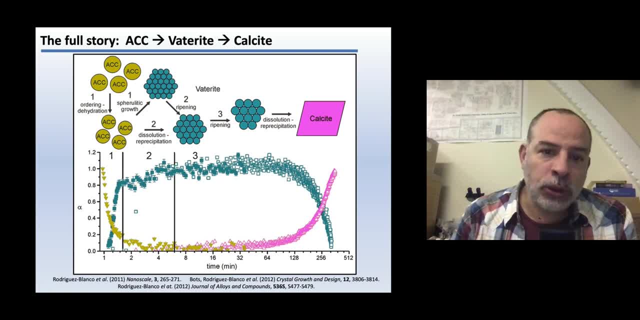 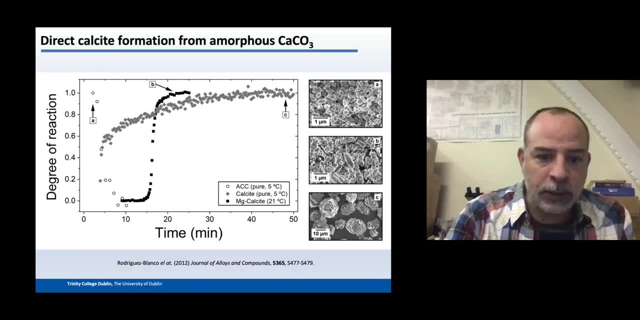 That would be much more complicated to follow using non-synchrotron-based techniques. Alright, And we have done the same, for example, for decrystallization of calcite from amorphous calcium carbonate. This is what you can see here. 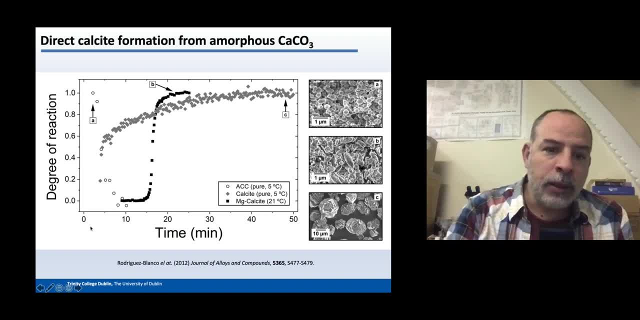 This is, for example, the decay of amorphous calcium carbonate And decrystallization of calcite- This grey chrome here- And also decrystallization of magnesium calcite. You see that all the process is gone in less than one hour. 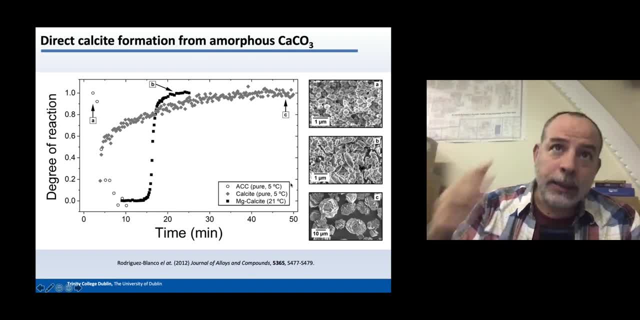 And we are done, And we are using low temperatures to decrease the kinetics of the reaction, And here magnesium calcite forms in less than 20 minutes at 21 degrees C. It will be very difficult to follow what is happening if we were not using synchrotron-based 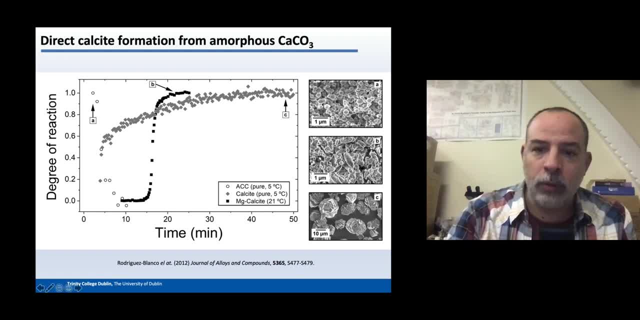 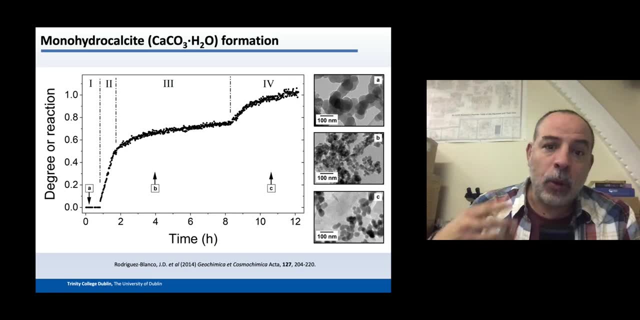 techniques. So this is what you see: Amorphous calcium carbonate forming calcite or magnesium calcite. Ok, In this case the process is a little bit slower, But we can use synchrotron-based techniques to follow this reaction with time and see. 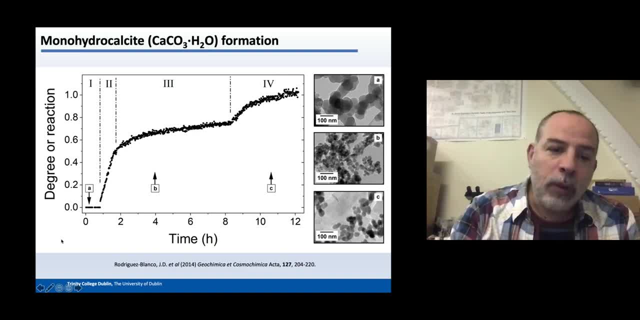 that we have two different decrystallization steps, In which we form monohydrocalcite, which is a calcium carbonate that contains some magnesium and water, And the first stage of decrystallization is quite quick, And then there are two slow growths that occur via Oswald-Rapening. 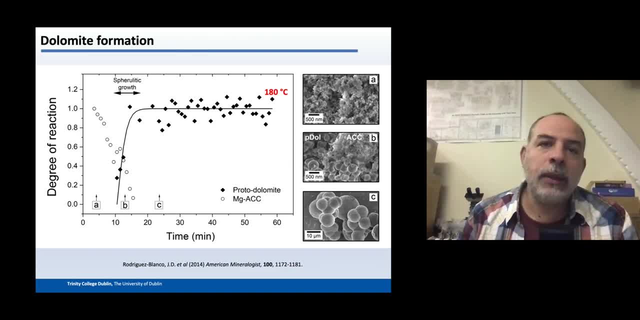 Something similar happens to dolomite. We need high temperatures to produce dolomite, And therefore it would not be possible to follow the decrystallization of dolomite without synchrotron-based techniques. You see here, at 130 degrees C. 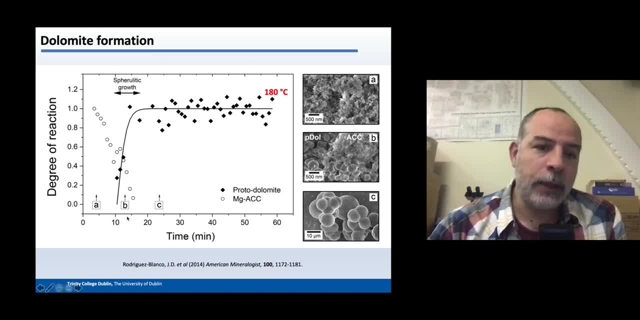 The breakdown of the amorphous phase, which is a magnesium-rich amorphous calcium carbonate, And the very quick growth of dolomite. This growth is essentially completed in less than half an hour. It would be impossible or very difficult to take samples from hydrothermal reactors and 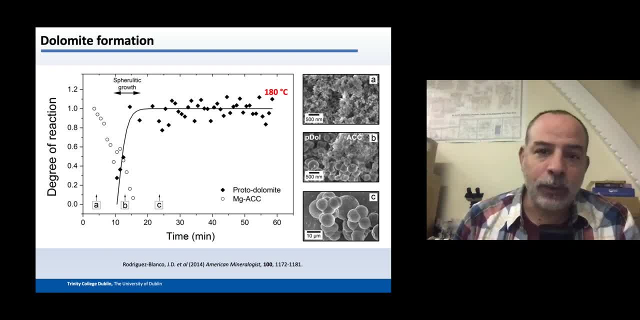 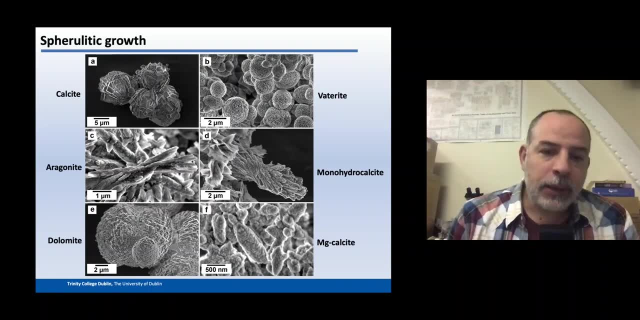 to study this at high resolution. We need synchrotron-based techniques to study this. What do we obtain at the end? What we have seen is that we, Every time any carbonate forms from an amorphous phase, the first stage of decrystallization. 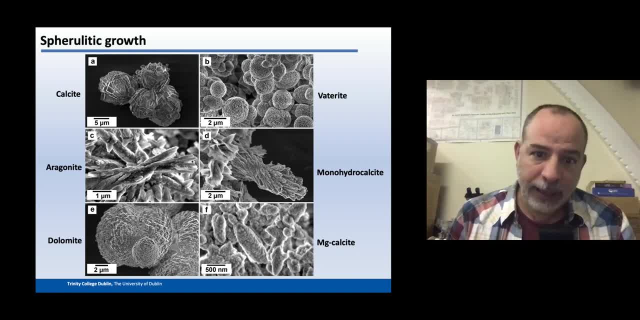 is usually translated into a spherical growth mechanism Because the amorphous phase breaks down very quickly, increases the supersaturation levels in the solutions dramatically and that is translated into a spherical growth of crystalline carbonates. And here you see some examples with calcite, aragonite, dolomite, batorite, monohydrocalcite. 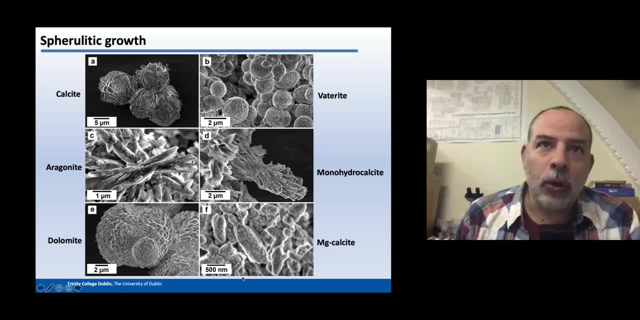 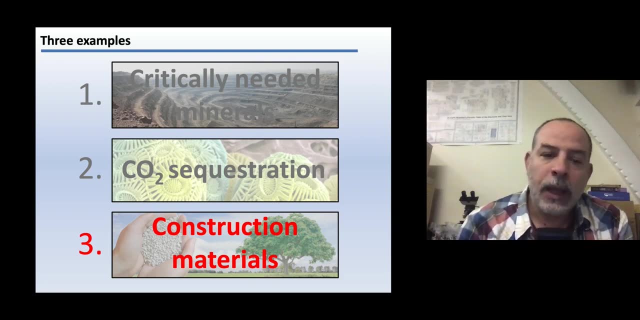 and magnesium calcite. All of them have grown by a spherical growth because of this quick decay of the amorphous phase at ambient or hydrothermal conditions. Now I'm going to focus on caustroxymathias, my third example, And in particular I want to talk about one mineral named gypsum. 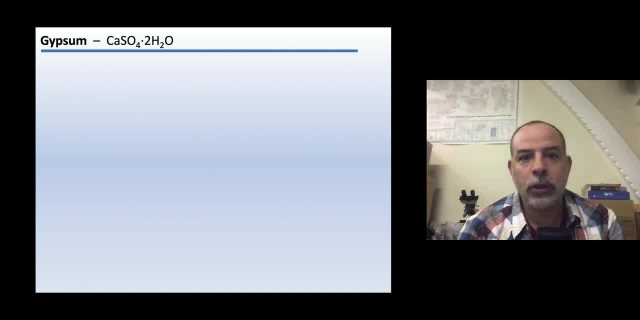 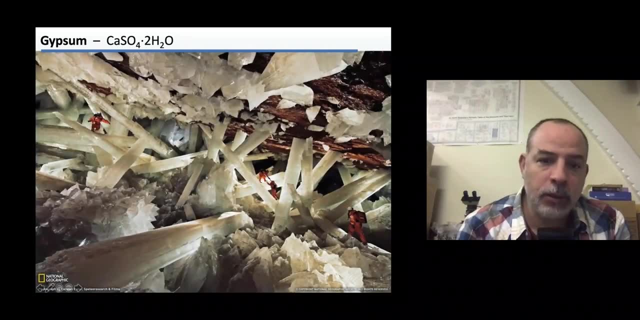 Gypsum is a quite common mineral. in nature It's a calcium sulfate with two water molecules, and it can be found in many places. Perhaps the most beautiful one is this one, Nica Caves in Mexico, where you can see single crystals of gypsum. but obviously gypsum can be found in many more places and is used by 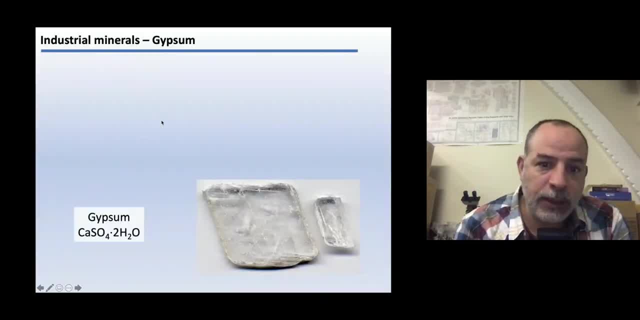 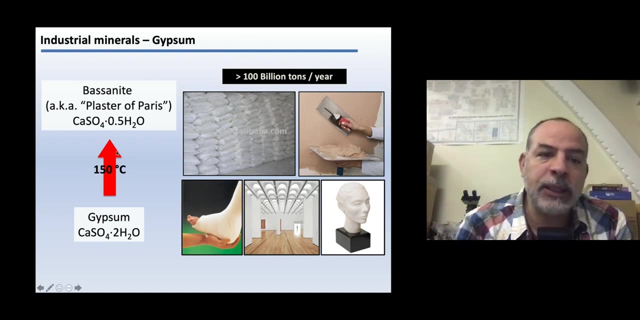 industry to produce one mineral which is essential, which is named basanite, also known as plaster of Paris. And, as you can imagine, there are many applications for plaster of Paris. Every year, billions of tons of gypsum are transformed into plaster of Paris by a simple 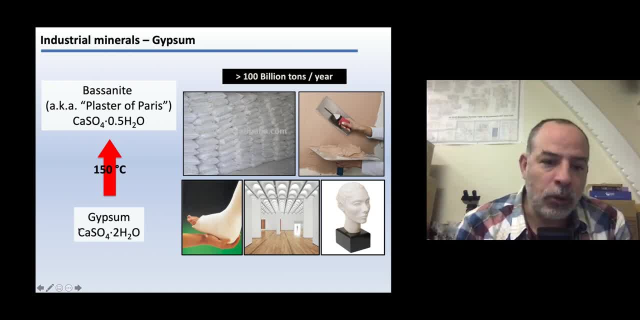 dehydration. So this gypsum loses 1.5 water molecules when it's heated up at temperatures of 150 degrees C, something that, as you can imagine, consumes a lot of energy and also produces quite a lot of CO2.. OK, so one of the research that was very fruitful a few years ago. it was a very nice collaboration. 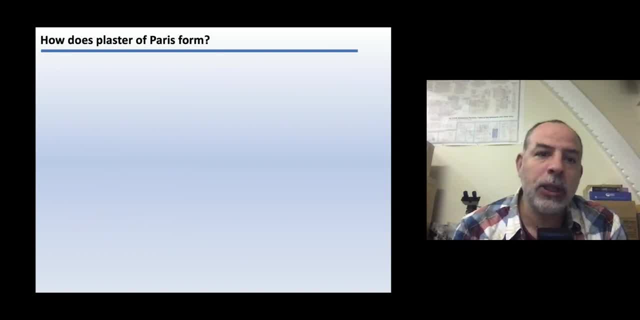 with people from different universities was to try to understand how plaster of Paris basanite forms. So initially we started. We thought that this crystallization pathway of plaster of Paris was going to be similar to the crystallization pathway in the calcium-carotene system, which goes from solution to anamorphous. 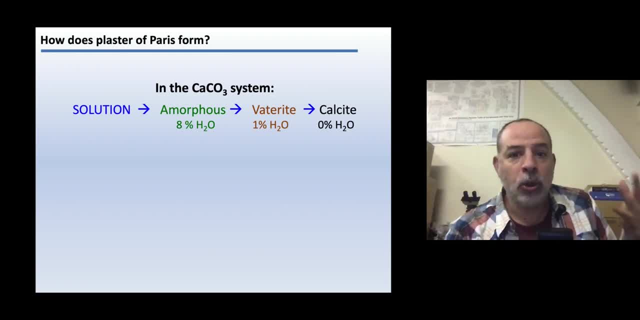 phase to butyrate and then calcite via dehydration. So we thought, OK, in the calcium-sulfate system perhaps we will go from solution to anamorphous phase, to gypsum and then basanite by losing water. And we were completely wrong. 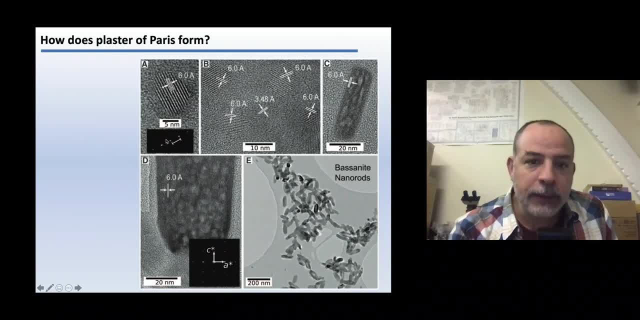 OK, It happens something completely different. What happens is that these calcium-sulfate phases don't grow via anamorphous precursor. They form crystals from the very early stages of reaction, And what happens is that some small nanoparticles made of basanite form from the very early beginning. 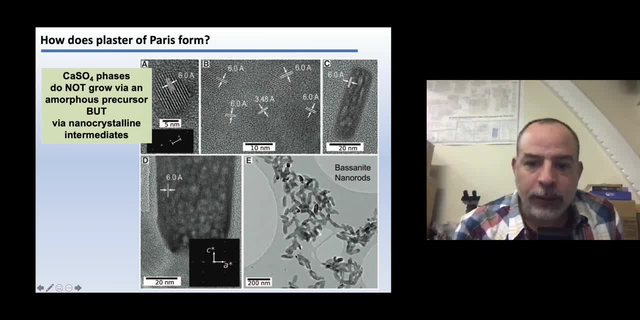 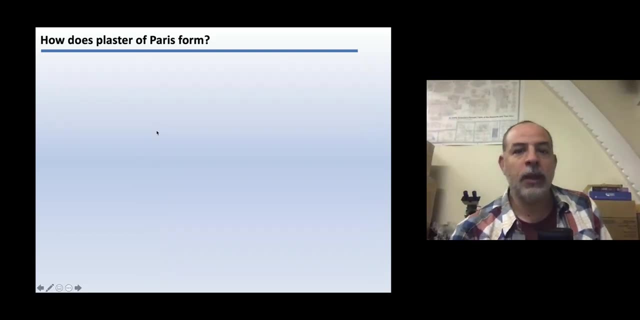 and they aggregate via oriented attachment, forming bigger rods of basanite, And then this basanite transforms into gypsum. So essentially, what happens is that gypsum forms via nanocrystalline intermediates. OK, We follow this using synchrotron-based techniques. 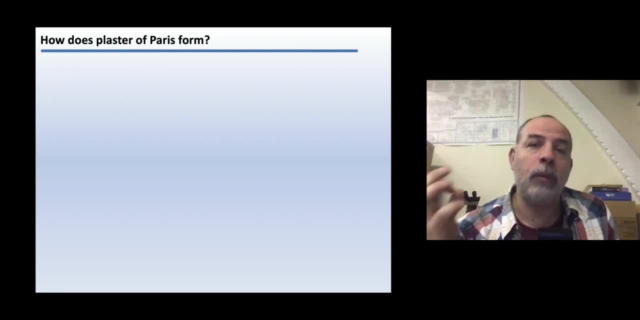 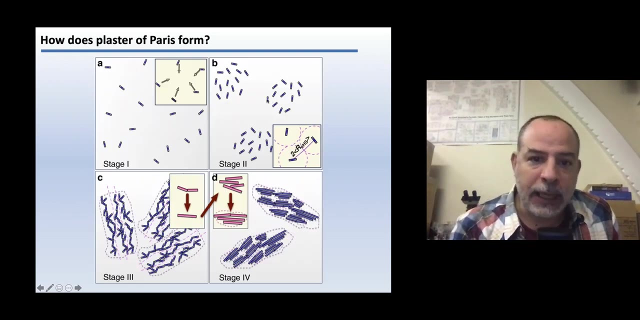 Without synchrotron-based techniques, it will be impossible or very difficult to follow these reactions, And what we found is that, yes, we go from solution then to basanite, then to this gypsum gaining water. OK, The process could be summarized by using a schematic diagram like this, in which you: 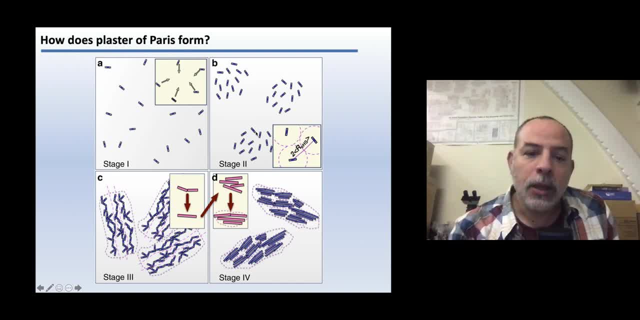 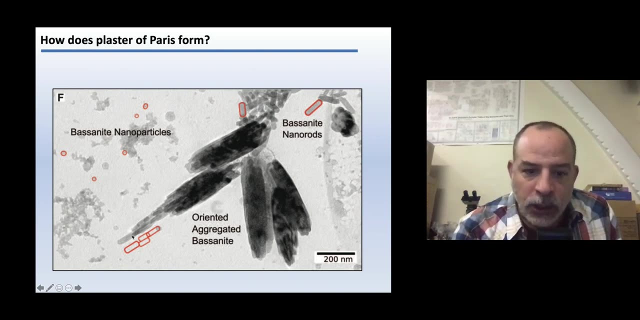 see the nanoparticles, nanorods, coming together via oriented attachments, which is depending on the surface energy and then later on transforming into gypsum. OK, And this is what you can see here: nanoparticles of basanite and then this oriented attachment. 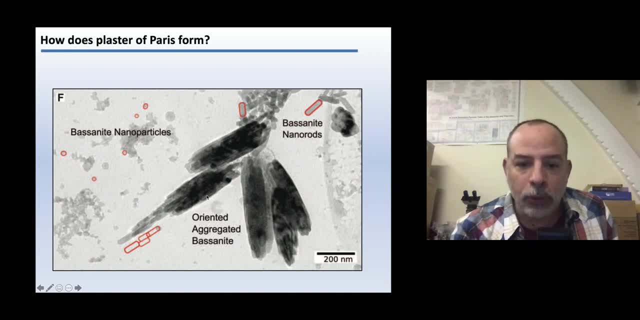 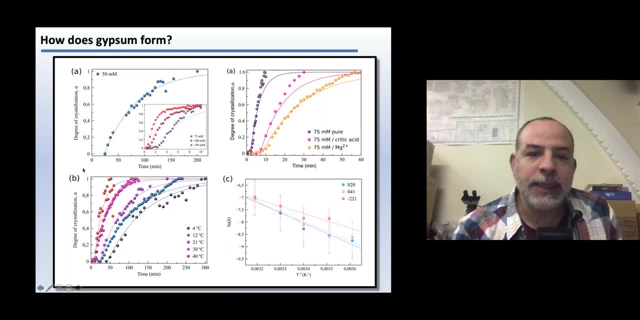 of these nanoparticles or these nanorods forming bigger basanite crystals, OK- And later on transforming into gypsum. So when we follow this by using synchrotron-based techniques, we could follow these reactions using different concentrations of calcium sulfate at different temperatures also. 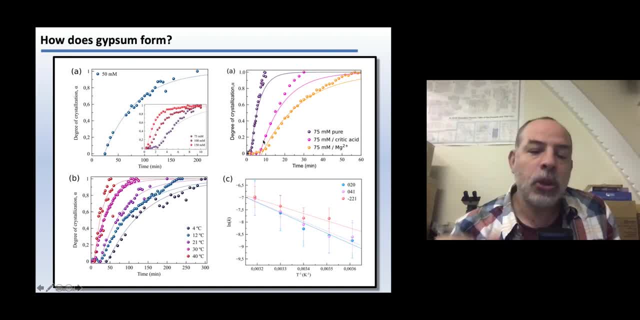 using organics and inorganics to try to see if it was possible to delay or to slow down the growth of basanite, which is something that happened. But as you can see here in time, things happened in less than a year. 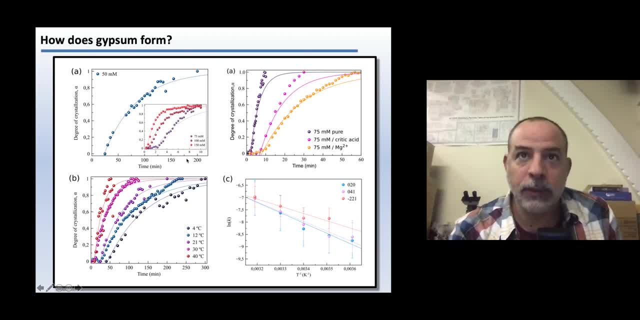 Less than a couple of hours. So this crystallization process is very fast, And we can only follow this by using synchrotron-based techniques. Otherwise it will be very, very complicated, And from here what we can get is the kinetics of the crystallization of nucleation and 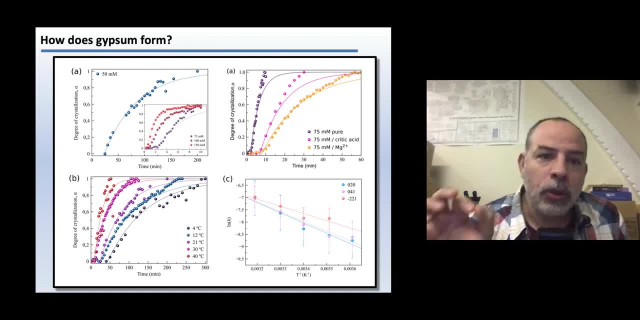 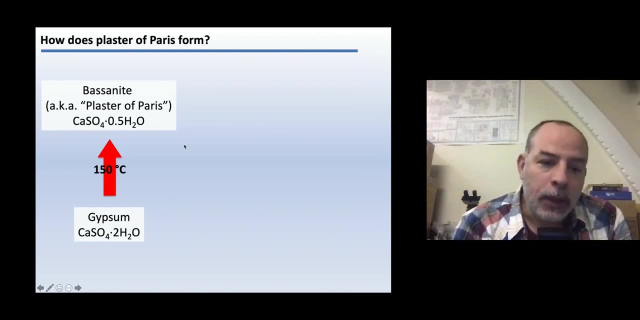 also the energetics of the reactions. OK, So this shows how useful synchrotron-based techniques can be to follow crystallization reactions. Otherwise, it will be essentially impossible to obtain so good data. OK, So what we saw is that, yes, we know that gypsum can be transformed into basanite at